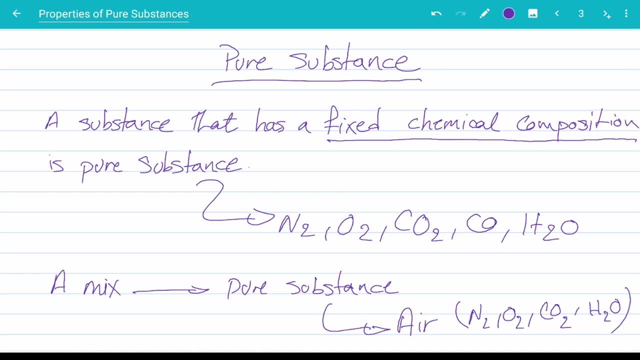 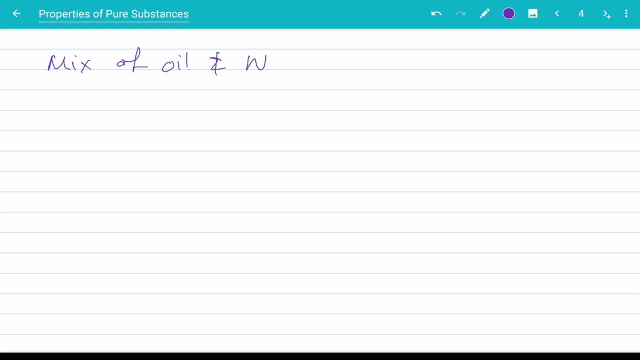 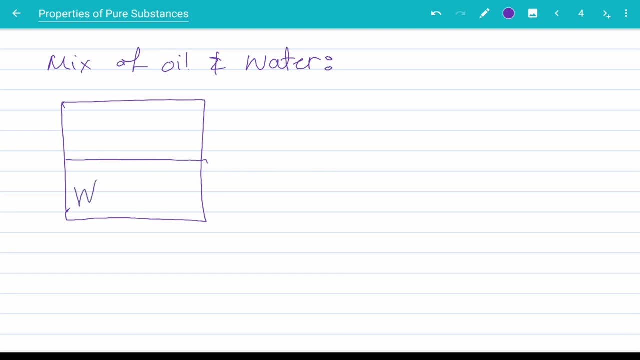 oil in it. So by experience we know that water stays on the bottom and oil stays on top. Now if I take a sample like this and check the chemical composition, I get 100% oil. If I do the sampling here, I get 100% water. And if I do something in the middle like this: 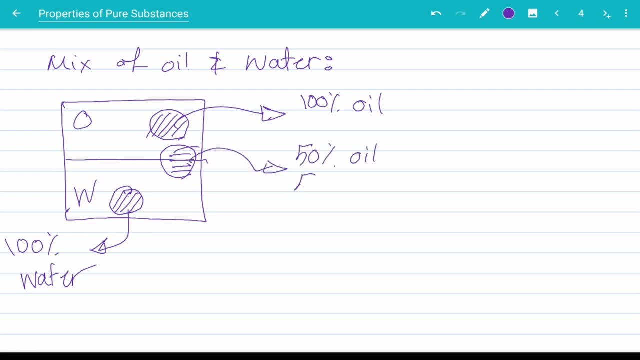 I'll get 50% oil and 50% water. Now, as you can see, the chemical composition at these three different locations inside this mixture are different, So it is not a pure substance. Now, a mix of different phases of a pure substance can still be a pure substance. 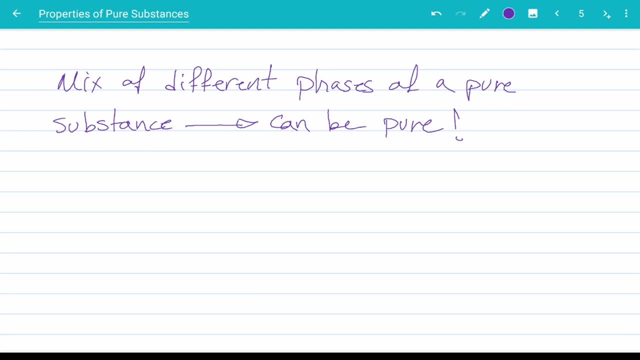 An example of this is water and water steam or water vapor. Now consider a container like this: we have liquid water here and then we have vapor or gas form of water on top. Now again, if we do three different samplings and check the chemical composition here in: 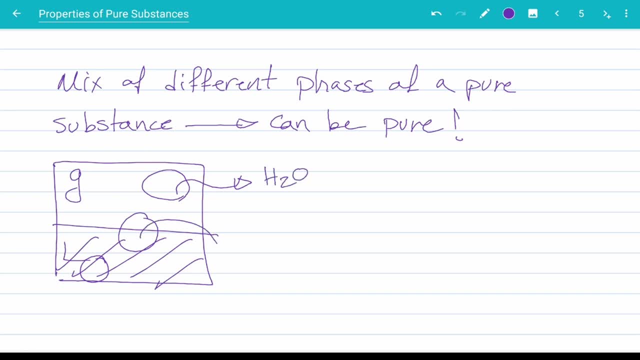 the gas form, the chemical composition is H2O, in the interface it is H2O and in the liquid it is H2O Again. so, as you can see, a uniform, fixed chemical composition throughout the tank. So it is a pure substance, although they have different phases. 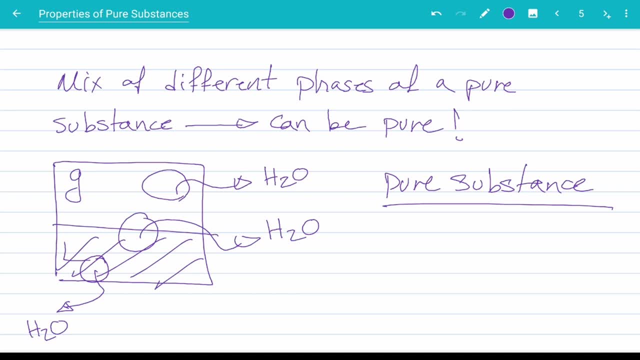 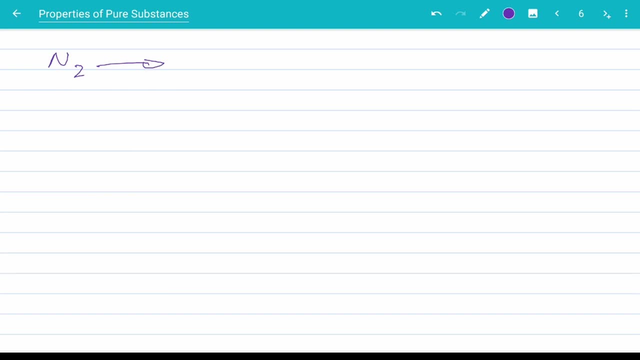 The same, however, cannot be said about air, for example. Now we know that nitrogen has a condensation point, or a boiling point, at minus 196 degrees per second. Oxygen, on the other hand, boils at minus 182 degrees Celsius. 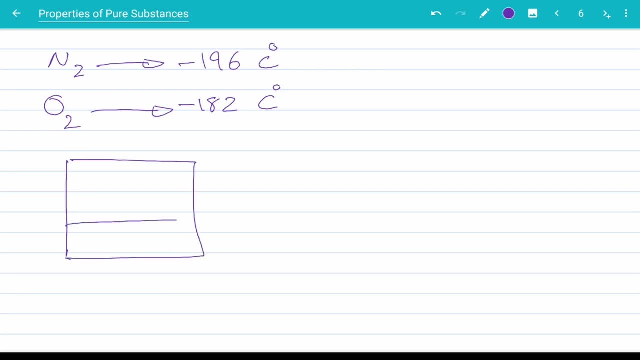 So let's consider a tank like this, where we are keeping some liquid air. So we have gas air here and liquid air here, And the temperature of this setup is minus 190 degrees Celsius. So if I take a sample from here, From here, the liquid is very rich in oxygen, right? 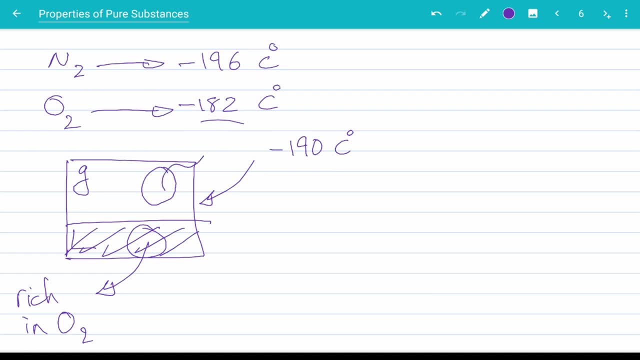 Because of the temperature. Now, if I take a sample from the gases form, it will be very rich in nitrogen. Now, as you can see, the chemical composition is not uniform or homogeneous between the gas and liquid phases, And so this is not a pure substance. 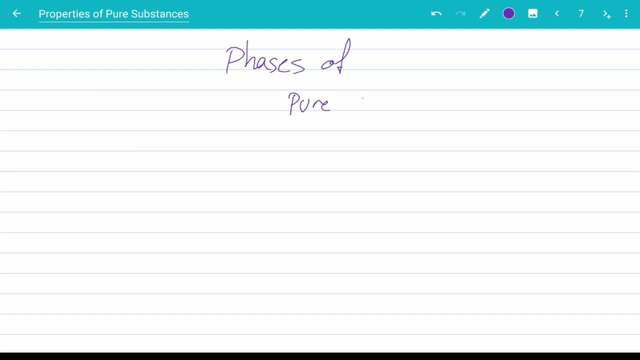 By experience we know different phases of pure substances. We know we have the solid, then we have the liquid and then we have the gases form. The molecules of a pure substance in solid form are seated in fixed positions with respect to other molecules around them, in some sort of a structured grid or lattice pattern. 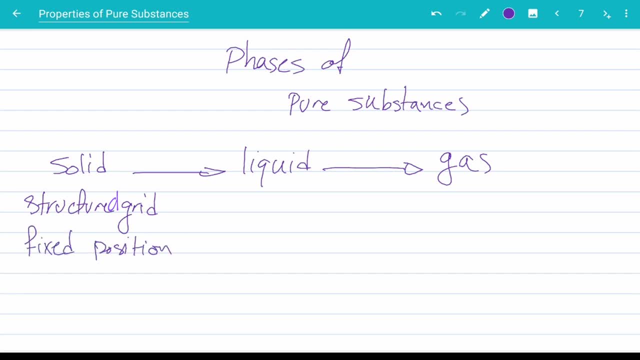 They cannot move out of their fixed positions, But they still can move. They still can vibrate and oscillate in their seats. The bonding forces keeping them in this grid are rather strong Now, if we introduce enough energy in the form of heat to a solid: the motion of the molecules. 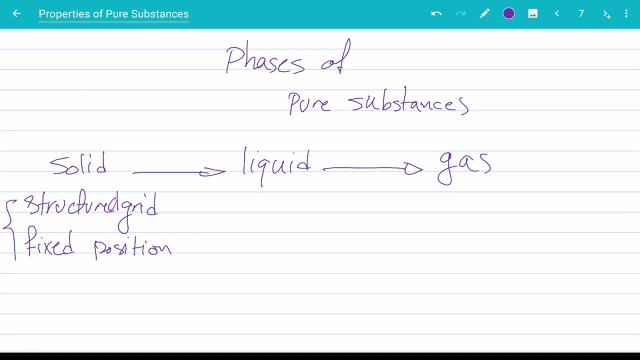 increases. the momentum of the molecules increases as their temperature rises, their internal energy rises and gradually they overcome the bonding forces that are keeping them as a structural grid. They go away. They go into the liquid form. Now, in the liquid form there is no structural grid, but the molecules are still bonded together. 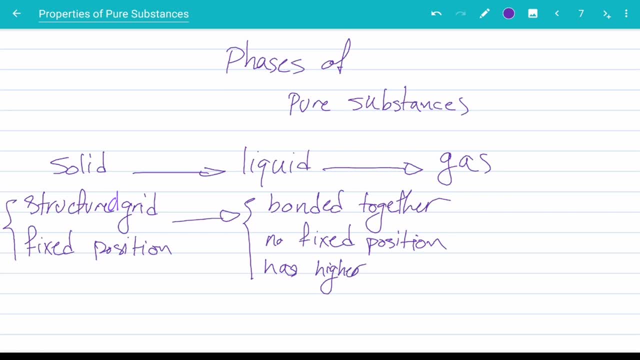 Because of all of the energy that we introduce to the solid to make it into the liquid. a liquid state generally has higher energy than solid. Now again, if we introduce enough energy in the form of heat, usually to the liquid, the molecules finally break free from that remaining bonding force and they go truly free. 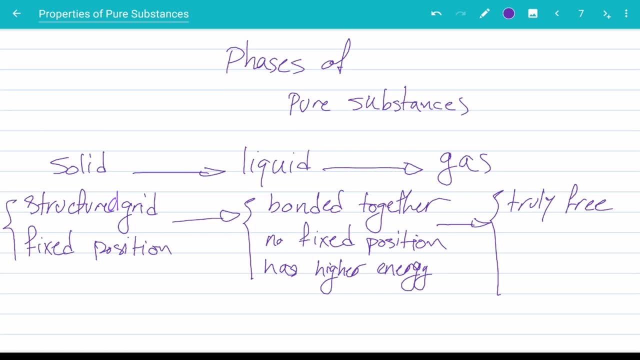 They can move in any direction that they want, with any velocity that they want. There is no structure in space and, again, because of all the energy that we introduce to the liquid to break the bonds, the gas form has the highest energy level between. 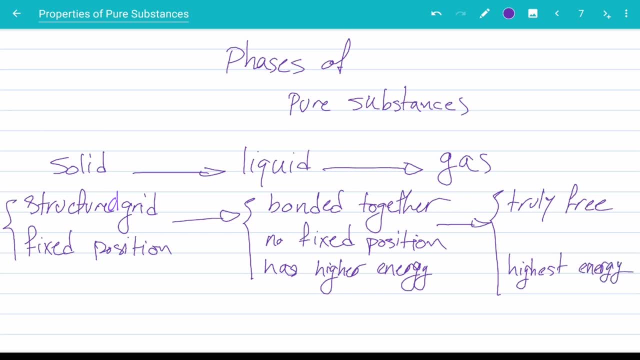 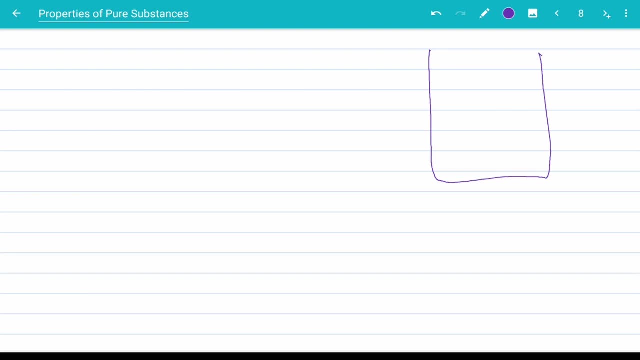 the three states. So that's it. Okay. so let's do a simple test. Let's consider a simple piston and cylinder system. The piston has no mass and the pressure outside is one atmosphere and we have water inside at 20 degrees Celsius. 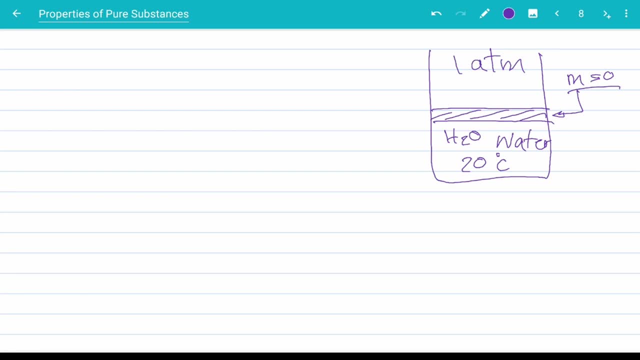 So this water is at room temperature and we know at one atmospheric pressure water boils at 100 degrees. So water at 20 degrees is not about to boil. Now, a liquid that is not about to boil or vaporize is called a sub-cooled or compressed. 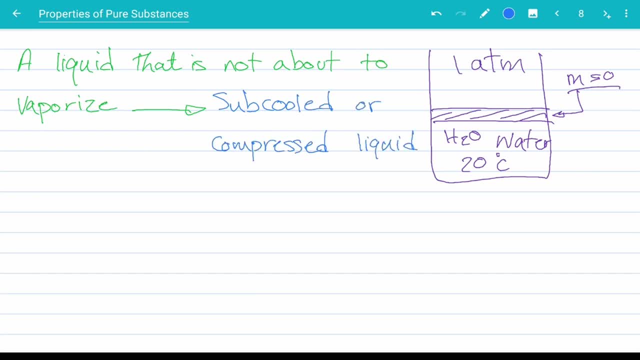 liquid. Okay, We are going to add heat for the piston. What do you see? And I want to adjust the temperature. What do you see to our system Now? because of the heat, the temperatures start to rise. let's say it goes to 40 and the water expands, right? because of the addition of heat. 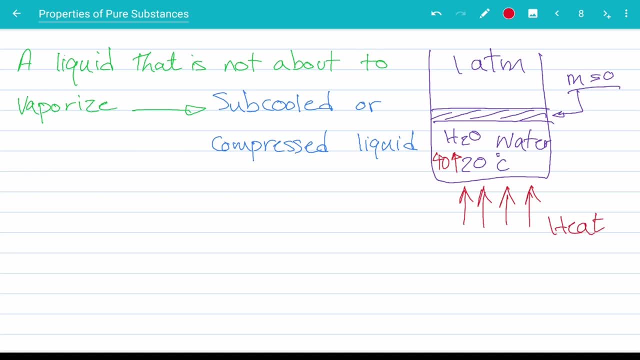 the water expands and the specific volume or the volume of our system expands as well, and the piston is now here, But the pressure is still one atmosphere and everything is still in liquid water form. We can continue to introduce heat until the water inside has expanded all the way it can and the temperature has. 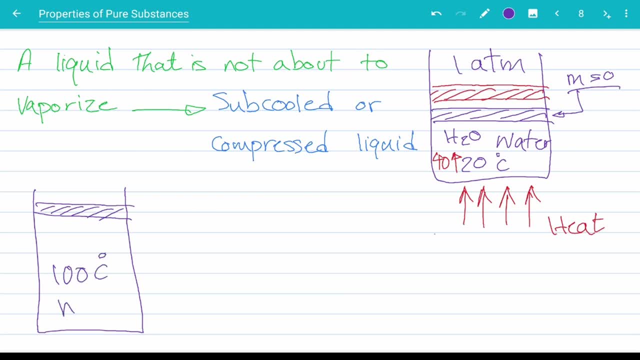 reached 100 degrees Celsius, We are still dealing with water in liquid form here. Now. here, if we introduce one bit more of energy in the form of heat, a single molecule or a single drop will break free from the liquid and go into the gas form. 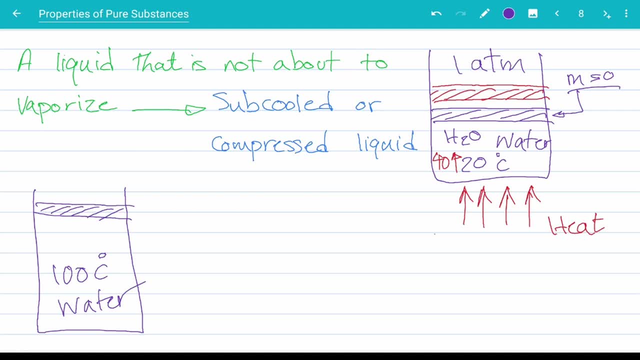 So this is the energy that we need to get out of the system. So this is the energy that we need to get out of the system. This liquid, here at 100 degrees Celsius, is about to vaporize Now, a liquid that is about to vaporize is called saturated liquid. 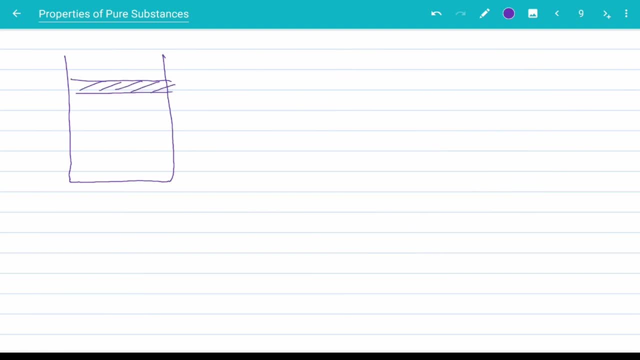 Okay, so we can continue to heat our system while the pressure is still one atmosphere and the temperature is still 100 degrees. but now a portion of our system is in liquid form, while the rest is in gas or vapor form. Now here we are dealing with a mixture of liquid phase and vapor phase, right, 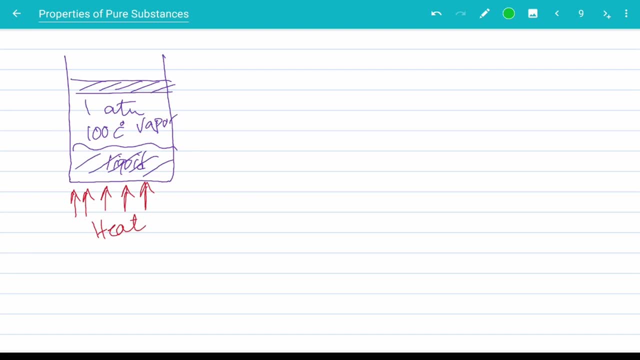 and they are now. this state here, where both liquid and vapor phases of water are inside the system, is called a saturated liquid vapor mixture. Okay, we can continue this and heat the system. Okay, we can continue this and heat the system. Okay, we can continue this and heat the system up to a point where every last 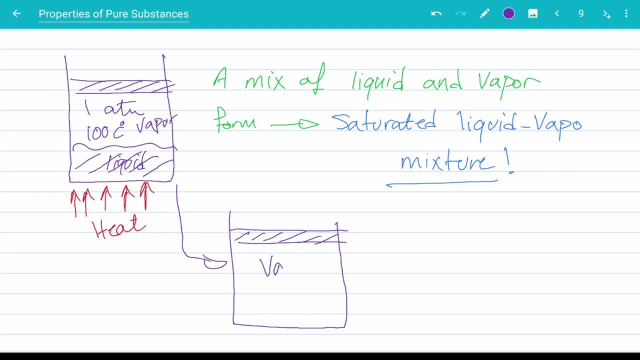 droplet of water has evaporated, so we have only vapor or gas form at 100 degrees Celsius. Okay now, in this situation, if we take one bit of energy or heat out of this setup, a single droplet or a single molecule of water will condense back into liquid form. 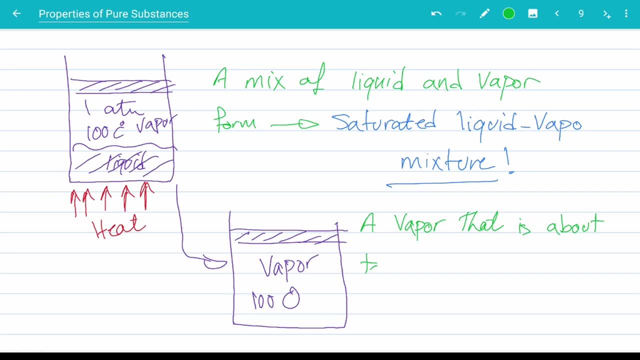 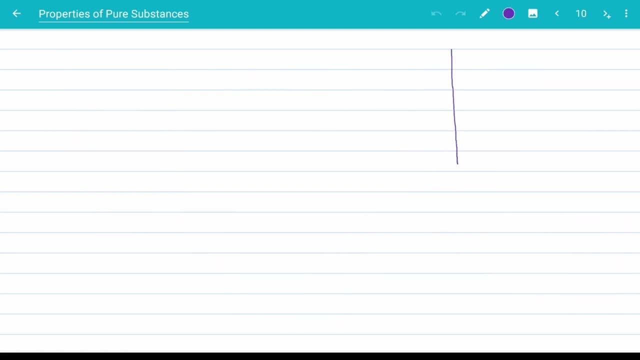 So this vapor is ready to condense Now. a vapor that is ready to condense is called a saturated vapor. Now we can again continue to heat up the vapor, and while the pressure is still one, And while the pressure is still one atmosphere, it will reach a temperature of, let's say, 150 degrees Celsius. 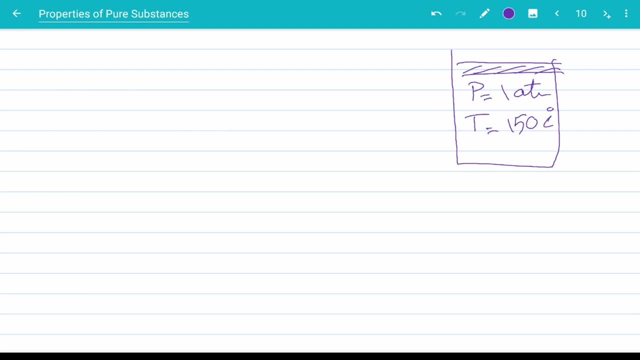 Now, here again, everything is in vapor form or gas form. we don't have any liquid. but the interesting thing about this is that So this vapor is ready to condense Now. a vapor that is ready to condense is called a saturated vapor. But the interesting thing about the state of our pure substance now is that this vapor 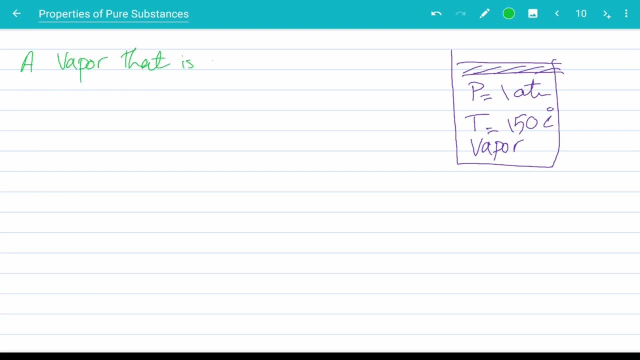 this gas is not about to condense. Now, a vapor that is not about to condense is called a superheated vapor. Now, based on this experiment and our previous knowledge, we know that at pressure of 1 atmosphere the water starts to boil at T equal to 100 degrees Celsius. right, 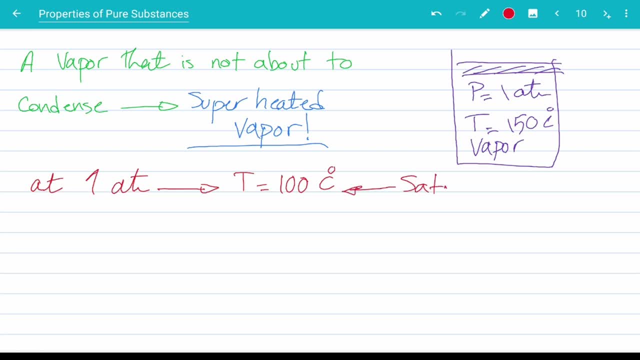 So for the pressure of 1 atmosphere, T equal to 100 degrees is called the saturation temperature And vice versa, for the temperature of 100 degrees Celsius, the pressure of 1 atmosphere is called the saturation pressure. So if you want to have a more official definition, at any given pressure, the temperature that 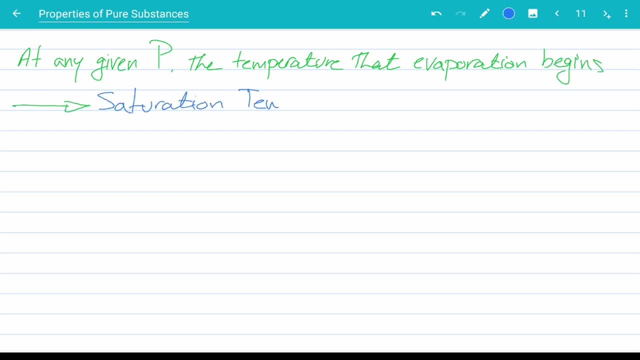 the pure substance is at is called the saturation temperature. The temperature that the pure substance starts to boil or vaporize is called saturation temperature, And likewise, at any given temperature, the pressure that the pure substance starts to vaporize is called the saturation pressure. 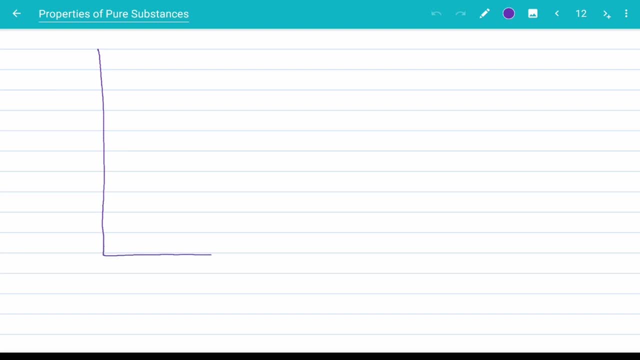 Okay. so if we want to draw the results of our experiment on a diagram, let's say on a temperature volume diagram or specific volume diagram, we get something like this. So we start our test with water at 20 degrees Celsius and then we started to add heat. 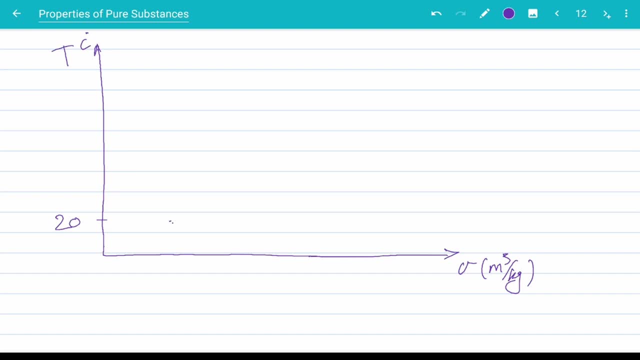 So the water started to expand right The specific volume, the initial specific volume, started to expand because we were introducing heat. Then we reached the temperature of 100 degrees where the phase change started. During the phase change The temperature remained constant right. 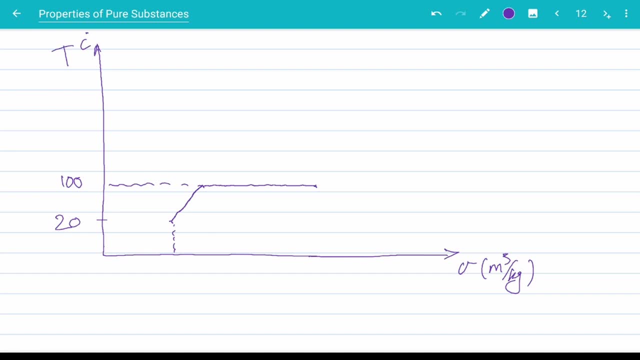 Until we reached the saturated vapor. From then on, the temperature rise again in the superheated region. So this area is called the compressed liquid. So let's go back to our previous test. The figure that we got area is called The superheated vapor. 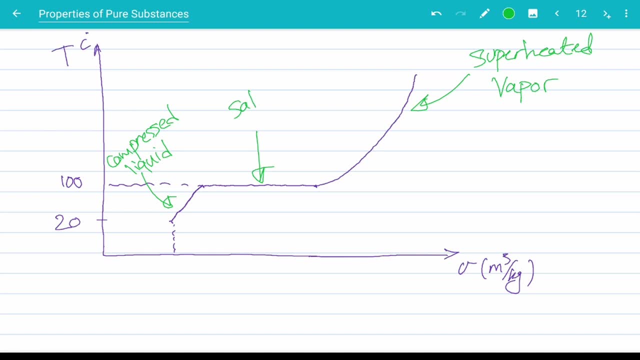 The area in the middle. this straight line is the saturation mixture or saturated mixture. This point here is the saturated liquid. This point here is the saturated liquid. This point here is the saturated liquid. This point here is the saturated vapor. This point here is the saturated vapor. 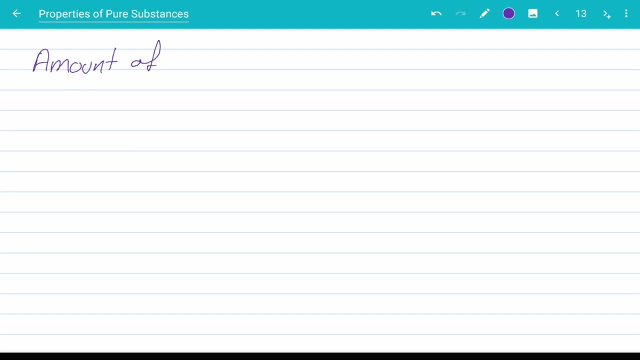 Now, we touched on this topic briefly before, but the amount of energy that is needed, that is absorbed or released during the phase change, is called the latent heat. So when you take your system to 100 degrees Celsius at one atmospheric pressure, the phase change has not started yet. 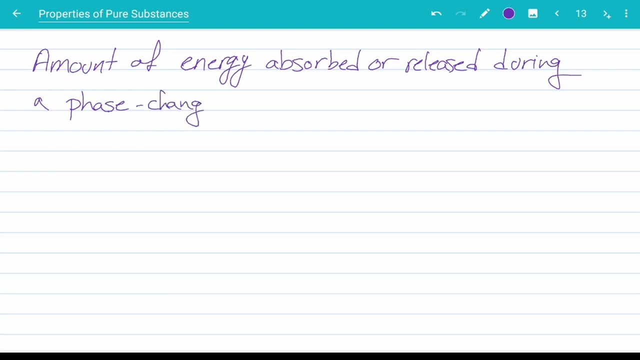 you keep adding heat to your system, while the temperature remains 100 degrees and the system goes from pure liquid all the way to pure vapor. Again, the temperature is not changing, but the phase is and it requires a lot of heat. All that heat goes into phase change and therefore it's. 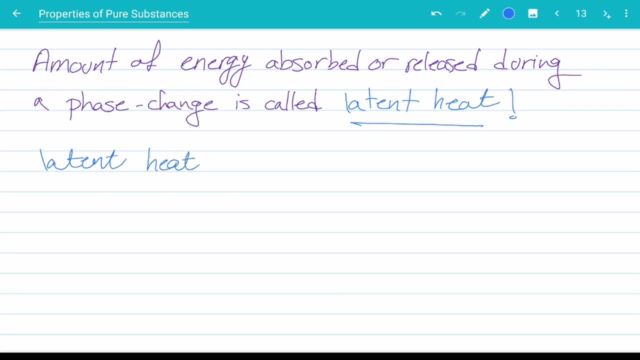 the latent heat or the hidden heat. Now, latent heat in general is a function of pressure and temperature of your system. So, for example, for water at one atmosphere, the latent heat of fusion, which is the melting or freezing process, is 333.7 kilojoules per kilogram, while the latent heat of 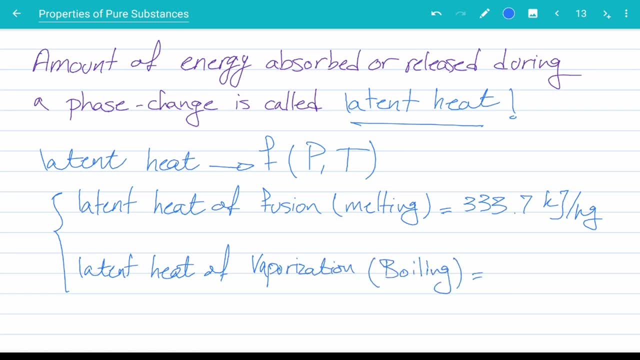 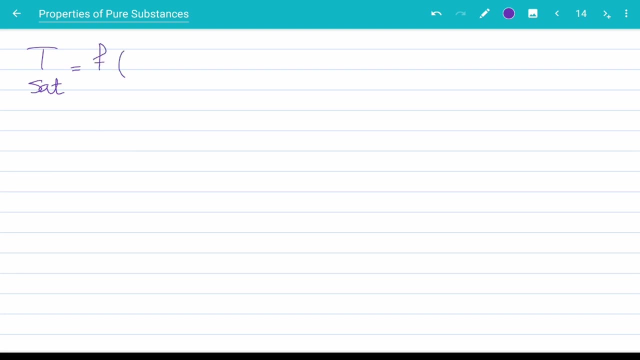 vaporization is 333.7 kilojoules per kilogram. So the latent heat of fusion is 333.7 kilojoules per kilogram. Now, one thing that you need to pay attention to is that the saturation temperature is actually dependent, or is a function, of the saturation pressure. What I mean by that? 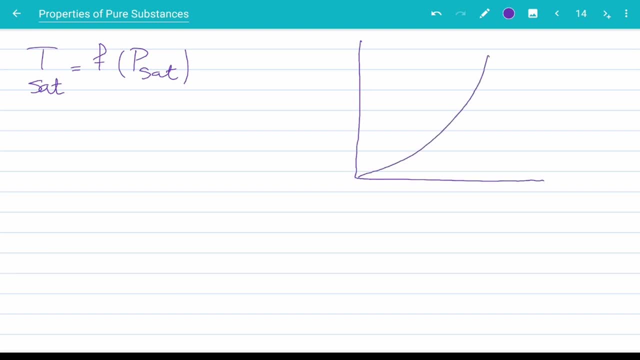 is they follow a trend. at least for water, you follow a trend like this, Where this is a saturation pressure and this is the saturation temperature. Now, here, let's say this is 100 degrees celsius, so the pressure is one atmosphere or 100 kilopascals. 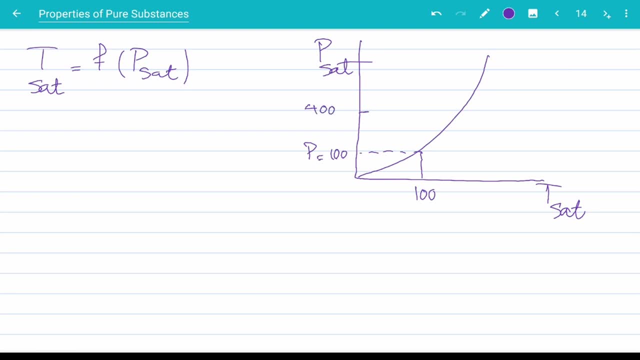 right, but at a pressure at, let's say, 400 kilopascals. the saturation temperature is about 143 degrees celsius. So, as you can see, the saturation temperature is about 143 degrees celsius And, according to the asker steps, they're dependent on each other. What this means is that, if we can 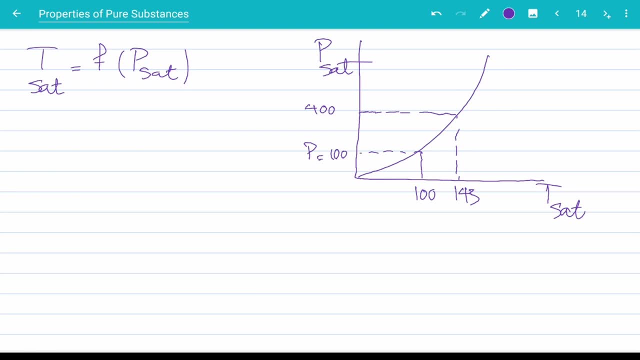 increase the pressure, we can increase the temperature at which the phase change happens. An example of this is what happens in a pressure cooker. Now, inside a pressure cooker, the pressure is higher than atmospheric pressure, And so the saturation temperature is also higher, right? So the food? 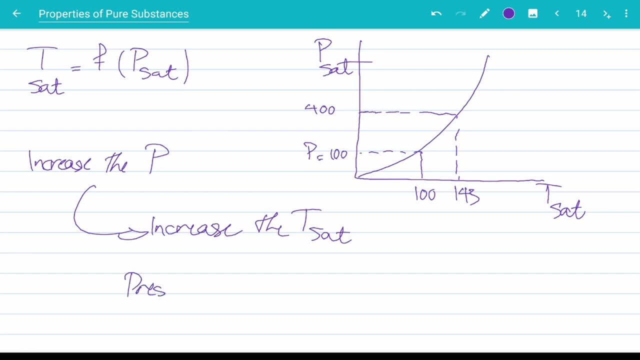 So the food is being cooked in an environment that the temperature is more than 100 degrees, while the water is boiling inside right, Whereas in a normal pot, because the pressure is one atmosphere, the maximum temperature that the water can get is 100 degrees. 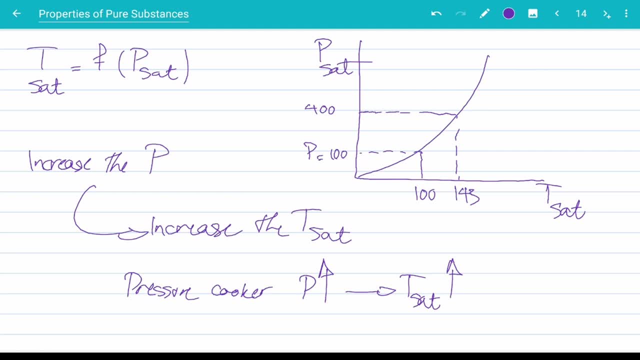 So a beef stew may take two hours in a normal pot, but take only 20 minutes in a pressure cooker. That's how it works. It increases the pressure, so it can increase the saturation temperature of the water, so it can increase the boiling temperature of the water. 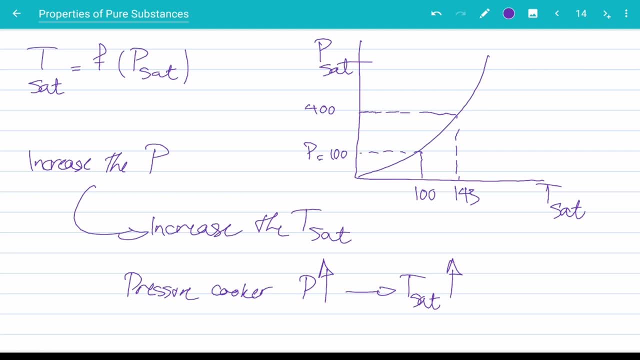 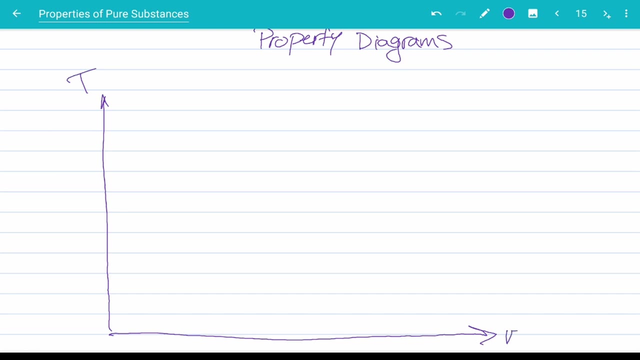 And so the temperature that the cooking happens at. Okay, let's talk about property diagrams. Let's go back to our first experiment. We drew the temperature of a specific volume And we started at 20 degrees For one atmosphere pressure. we had a curve like this: 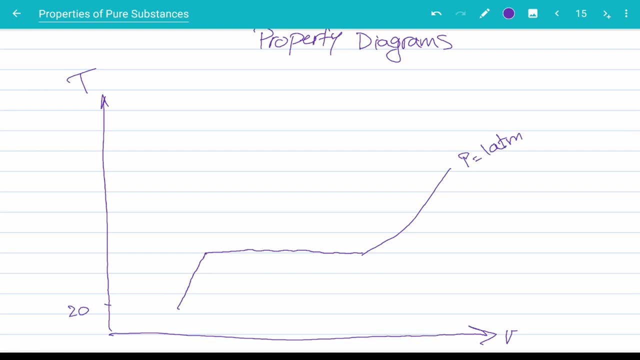 Now, if we increase the pressure- let's say we increase it to one megapascals- what happens is that, because of the additional pressure, our liquid, at any given temperature, has smaller specific volume. because it's been under more pressure, it's been a bit more compressed. 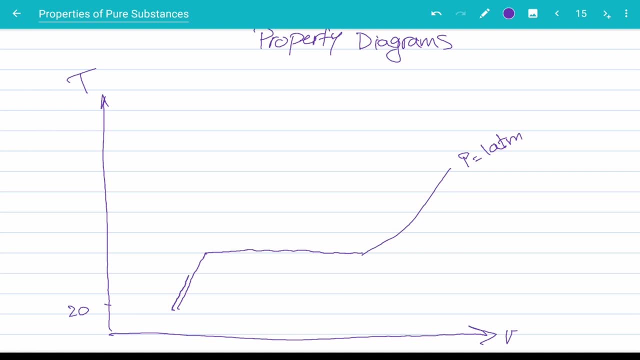 so it has less specific volume. So at 20 degrees we start at a smaller specific volume. So at 20 degrees we start at a smaller specific volume. So at 20 degrees we start at a smaller specific volume. And now, because the saturation temperature is a function of pressure, we reach the saturation. 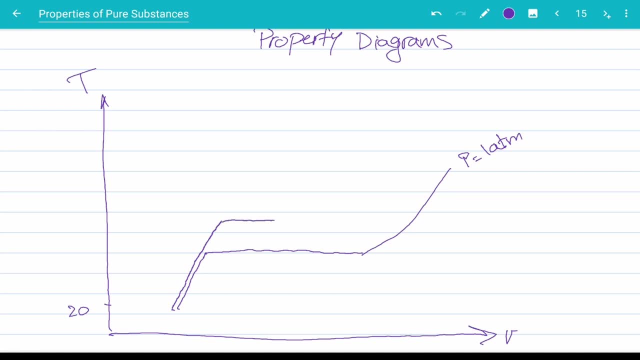 liquid state at a higher temperature, Then the phase change happens And then we go into the superheated region. Now we can continue this with higher pressures and every time we get a bit higher where the phase change starts. Something that you need to pay attention to is that this line, which represents the phase, 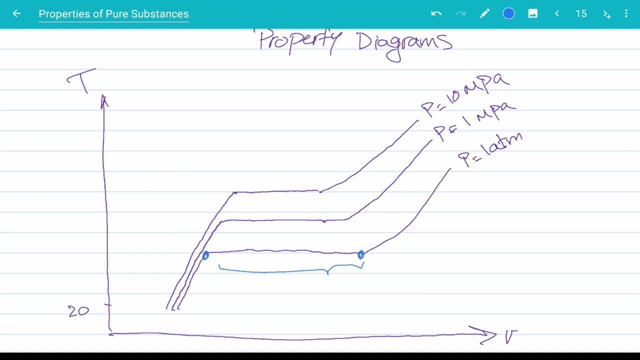 change phenomena. so here everything is liquid, here everything is vapor. So this line- we call it the saturation line- shows the phase change process. Now, as you increase the pressure, as the pressure goes higher, this line gets higher, smaller and smaller. The saturation line gets smaller until we reach a pressure. 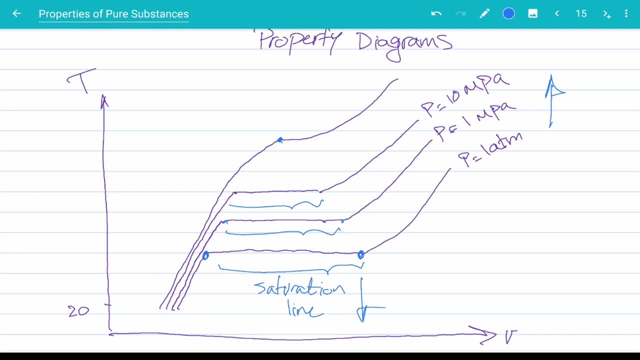 where the line reduces to just a single point. At this point saturated liquid and saturated vapor are the same. There is no phase change process. This point is called the critical point For water. the properties at critical point are listed here. The critical pressure of water is 22.06. 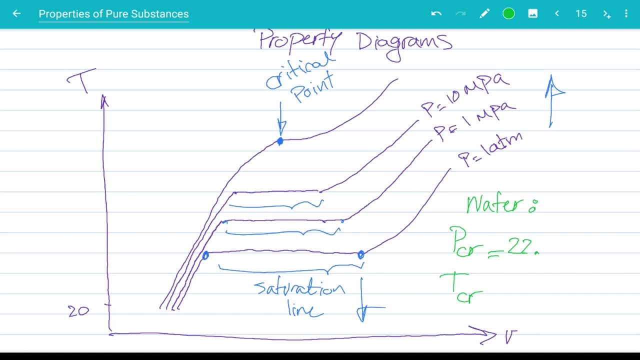 megapascals. while the critical temperature is 373.95 Celsius, The corresponding specific volume is also called critical specific volume and for water it is 0.003106.. We can have processes with pressures higher than the critical pressure and you can still get them on this diagram, but for these processes, 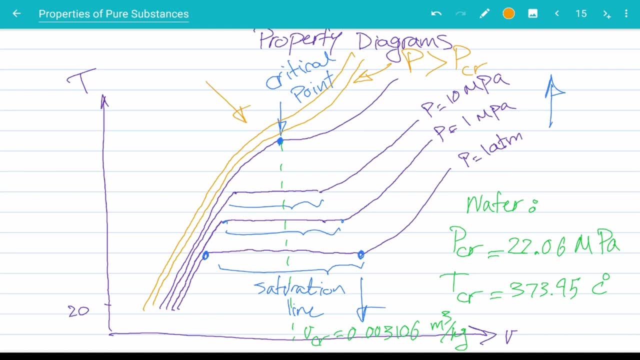 so these have pressures larger than critical pressure for these processes. there is no phase change. there is no obvious, no obvious phase change happening. So we have liquid up until a point and then we have vapor from then on, But that exact point. 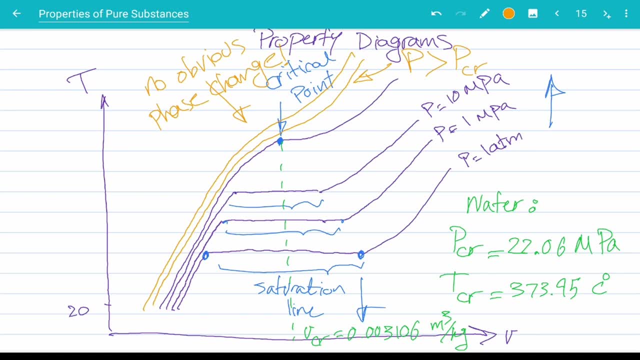 where the liquid turns into vapor cannot be pinpointed, cannot be known. It just happens. But as a rule of thumb, anything that falls on the left-hand side of the critical point, we treat it as compressed liquid, And anything that falls on the right-hand side of critical point, we treat it as superheated vapor. 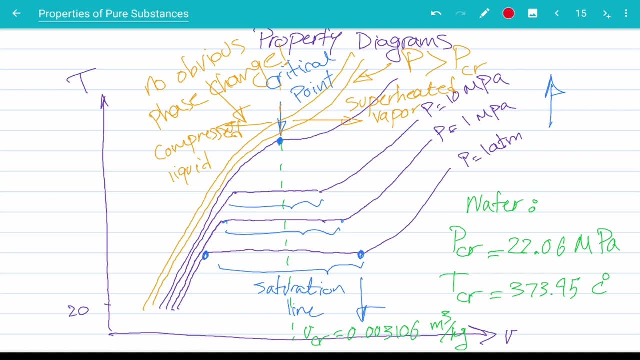 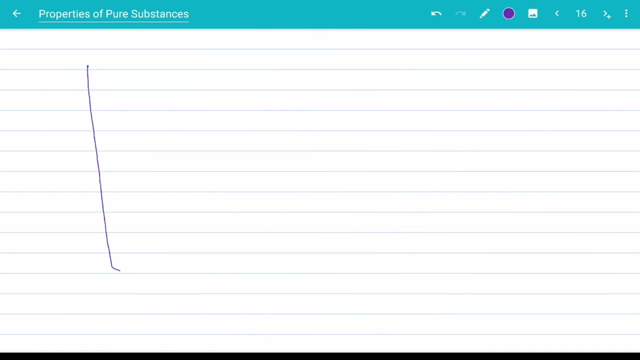 Now, if we connect all the saturated liquid points and then connect them to all the saturated vapor points, we get a dome like this. Now, let's clear this up in another page and we can continue talking. So this is still our temperature versus specific volume diagram. 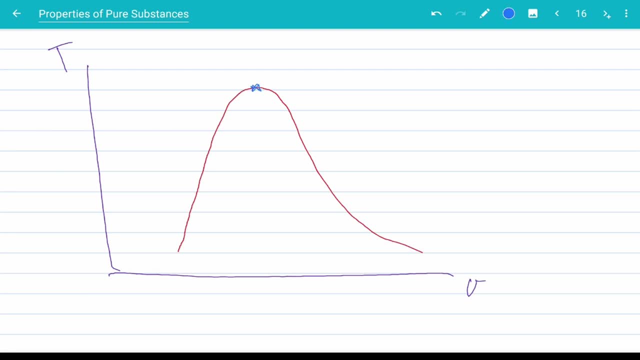 and this is our dome. So up here is the critical point. These are pressure constant lines and this is the temperature constant line and this is the temperature constant line. So this side of the dome is called compressed liquid side. Anything on the dome is saturated liquid. 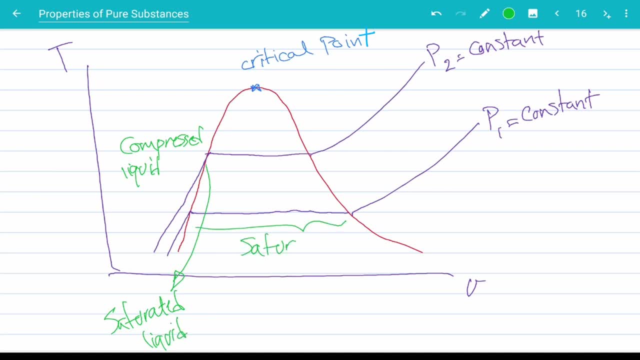 The area in between is a saturated mixture. The area in between is a saturated mixture. Anything on this side of the dome is saturated vapor And, of course, anything right-hand side of the dome in this area is superheated region. Now this is called a T-V diagram. 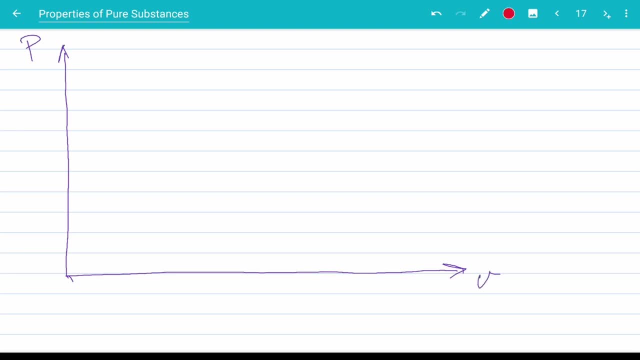 We can draw the data on another pair of paper. We can draw the data on another pair of axes. We can put pressure and specific volume here and then get more or less the same dome. Now in this diagram, the constant temperature lines are like this: 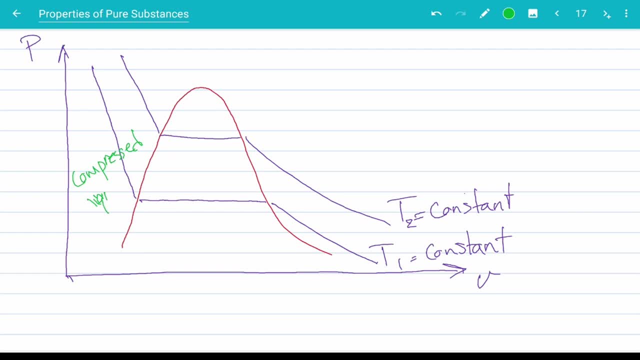 Again, this side is compressed liquid. This is the critical point. This is the temperature constant line. This is the temperature constant line. This is the critical point. This side is superheated region. This area is saturated mixture. Any point on this side of the dome line is saturated vapor. 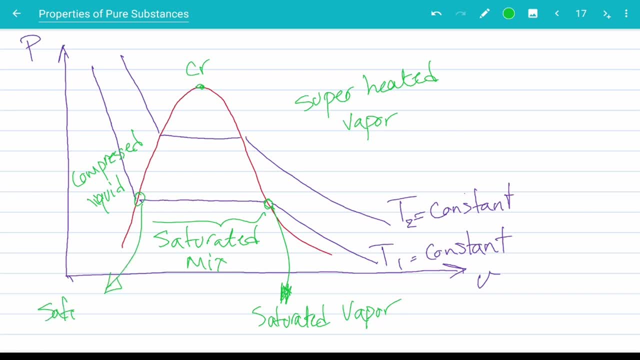 And anything on this line is saturated liquid And anything on this line is saturated liquid. This is a P-V property diagram. Now, these diagrams- the PV and the TV diagram that we discussed so far- are really focusing in this form, are really focusing on the phase change and phase equilibrium between the liquid. 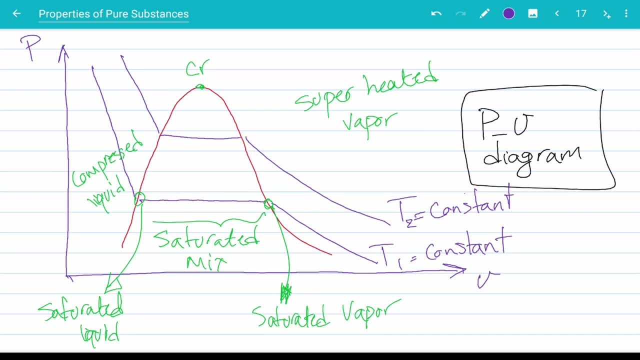 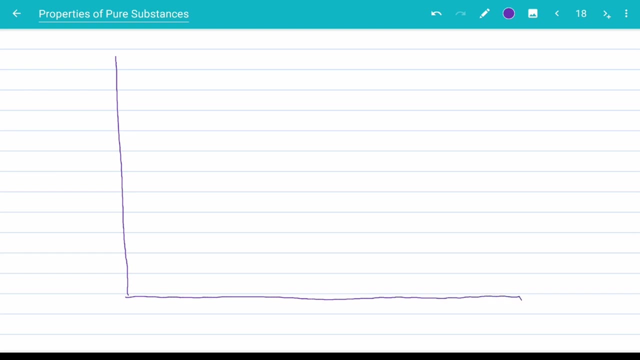 and the gas. We can also add solid to these diagrams because there is a phase change between solids and liquids, and solids and vapors as well, but I'm not going to do that because I want to keep this simple. We can talk about the phase change of solids with liquids and gases in another diagram. 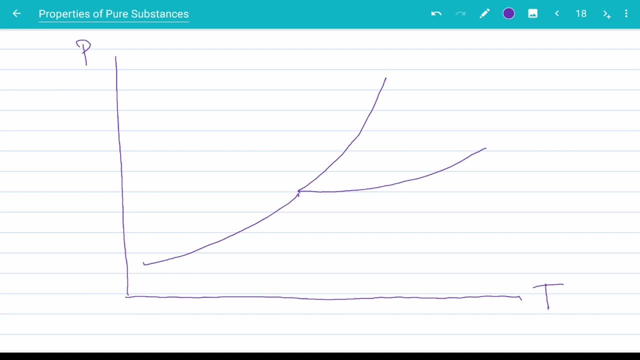 in a P-T diagram. So let's take a look at a P-T diagram. So this line here is the vaporization and it ends on the critical point where we saw in the PV and TV diagrams. So this is the critical point. So if that is true, then this area down here is vapor. 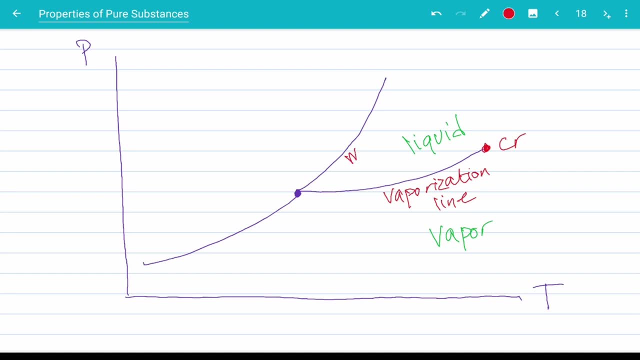 Okay, And the area here is liquid. This line here is the melting line. This side over here is solid. Now, vapor and liquid, they have a vaporization line. Liquid and solid have a melting line, and solid and vapor have a sublimation line. 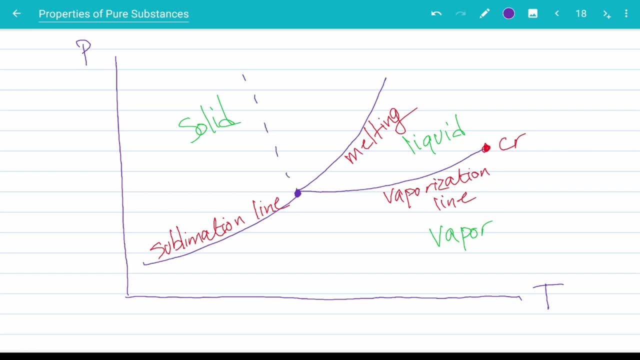 Now I'm going to add another line here. This is also melting. Now, the difference between these two melting lines is that this one is for normal substances, or the ones that contract on freezing. This line over here is for substances that expand upon freezing, like water. 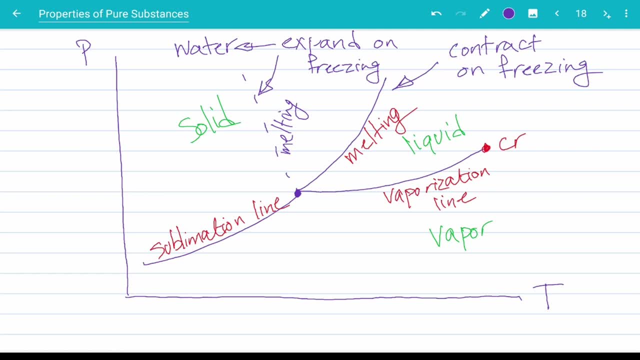 Okay, So let's take a look at this. So it shows that at different pressures and temperatures we can have different forms of a substance On a vaporization line. on a right pressure and a right temperature combination, we can have a mixture of both liquid and vapor forms. right? 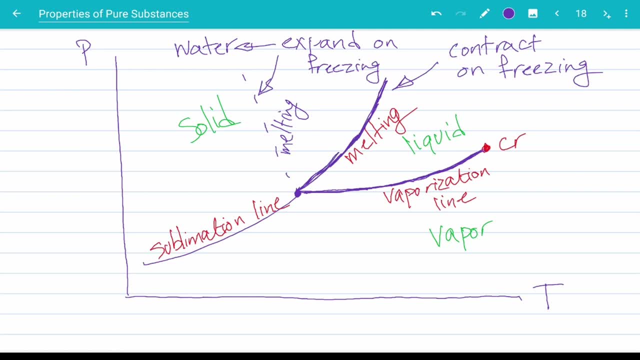 With the right combination of temperature and pressure, we can have both phases. We can have both phases of solid and liquid at the same time. And again, with the right combination of pressure and temperature, we can have both phases of solid and vapor at the same time. 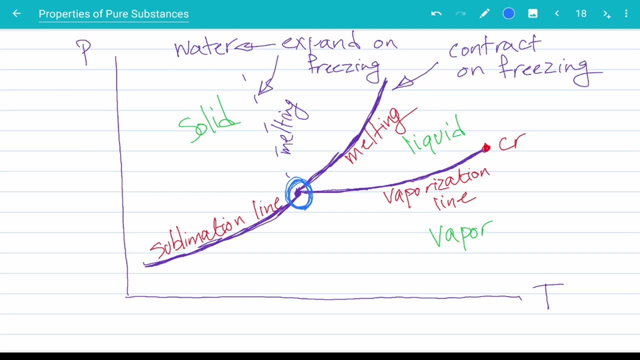 There is this point in the middle, however, that at certain pressure and temperature combinations we can have all three phases. Now this point is called the triple point of a pure substance. Now for water. triple point is achieved at 0.6117 kPa and temperature of 0.01°C. 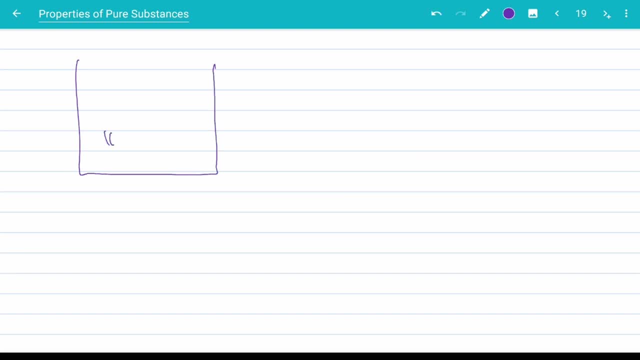 Now what I mean by having all three phases. let me give you an example. Now, in a system where the temperature is 100°C, we can have a situation that half of the container is liquid. Well, the other half is liquid, The other half is vapor. 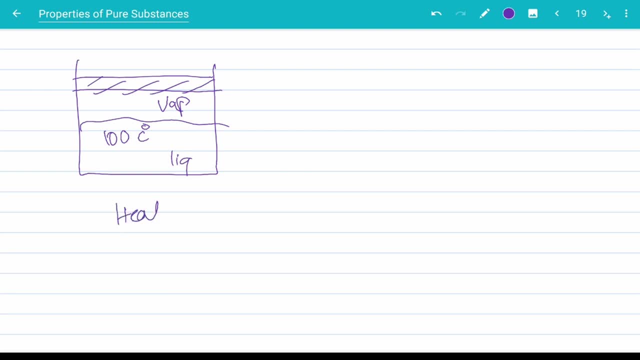 If we do not add any heat and we insulate the entire system, then the vapor and the liquid at 100°C will remain there. They will stay in a phase equilibrium. okay, Now, if we add more heat, sure, the liquid goes into the vapor, and if we take heat out? 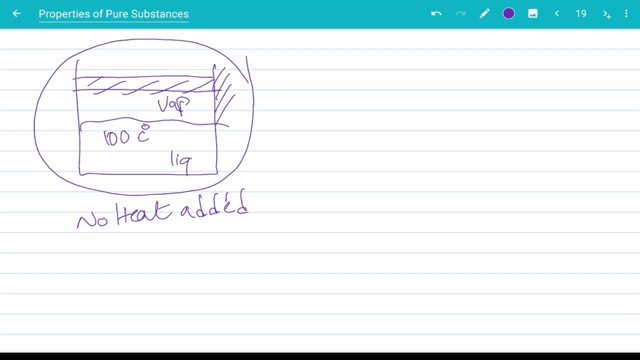 of the system. sure, the vapor condenses back to liquid, right. But if you put some ice inside of this as a third phase, if you put ice in, that ice cannot stay in. It will melt down and condense some of the vapor back into the liquid. 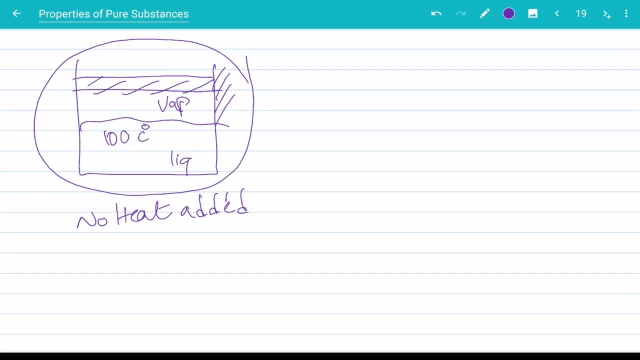 Alright, because ice absorbs the energy and melts down at 100°C. So the pressure here was one atmosphere. Now consider the same situation. Here's another situation. Look at the quería. Look at the point of surface edge is 0.6117 kilopascals and the temperature is 0.01 degrees Celsius. 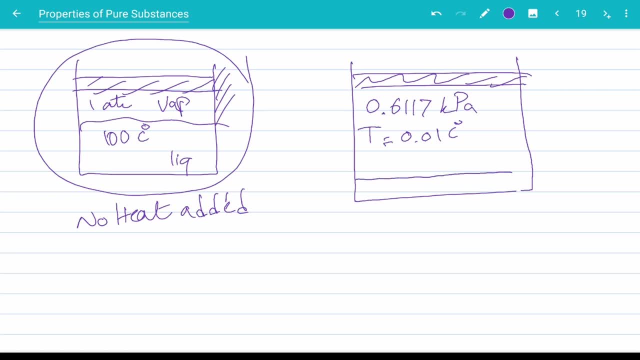 Then I can have a layer of ice topped with a layer of liquid water and topped with vapor. Again, let's say everything is insulated and no heat is coming in or out of system. If that is true, then this ice, this liquid and this vapor can all. 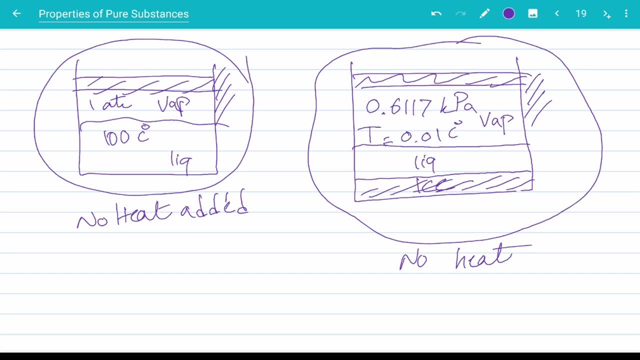 coexist in the same system at the same time, or in other words, they will be in a phase equilibrium together. So that is a triple point for you. Triple point is a situation where all three phases of a pure substance can be together in a phase equilibrium. 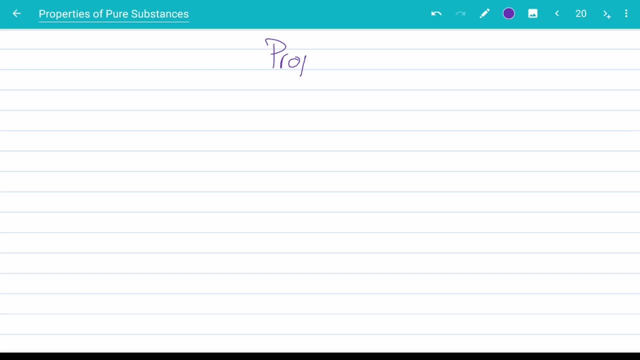 Okay, now we are ready to talk about property tables and reference states. For most substances, the relations among thermodynamic properties are too complex to be expressed by a single equation, So therefore these properties are usually given in table forms. Now here's an example. Now this is a property. 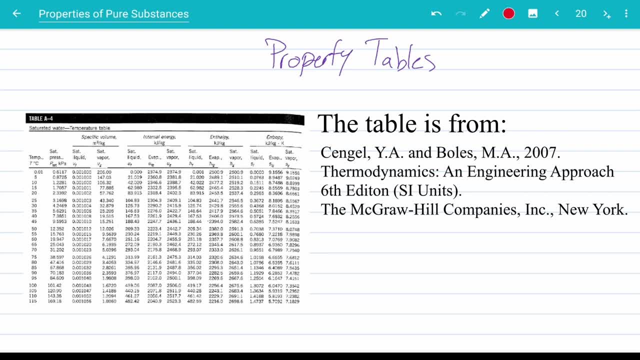 table. As you can see, various properties of water is given based on the saturation temperature or based on the temperature Right. So this column here is the temperature, this column is the saturation pressure and these columns are showing the internal energy. these are showing 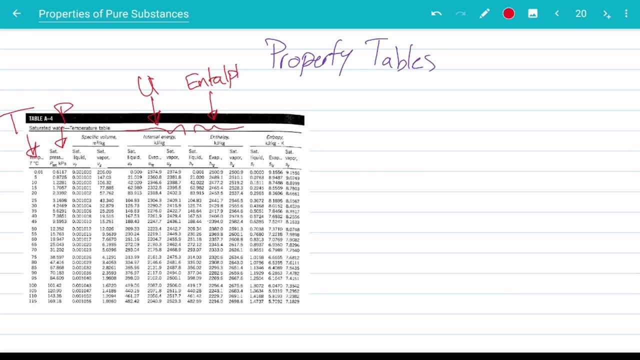 enthalpy and these are showing entropy. So enthalpy is internal energy plus pressure times, a specific volume. We show it with H and this is the equation for it. Now we'll talk about enthalpy in future videos, but enthalpy usually shows up when dealing with control volumes and 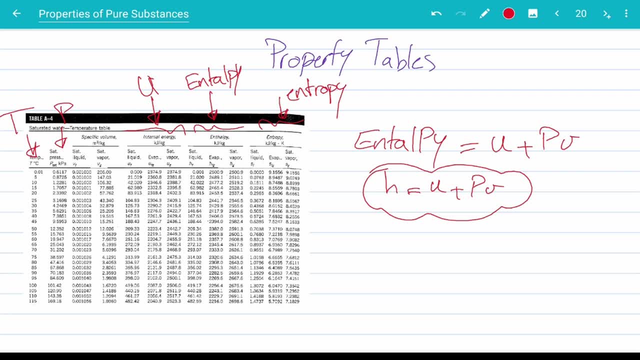 the situations where a fluid is flowing in and out of a system. But for now let's just take the definition of enthalpy as the summation of internal energy and pressure times a specific volume. Now this equation, this form, has a unit of 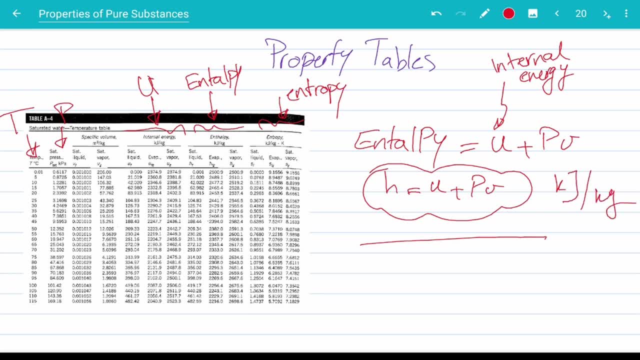 kilojoules per kilogram. We can have the extensive one, as in capital letter H is capital letter U plus P volume, and the unit will be kilojoule. Okay, with the definition of enthalpy out of the way, let's focus on the table, As you. 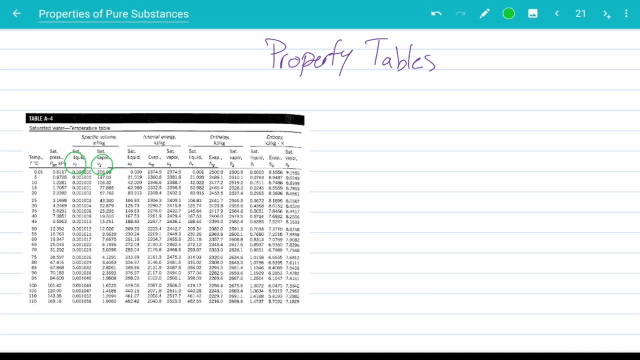 can see, there are two specific volumes listed for each temperature. One of them has a subscript of F, the other one has a subscript of G And for the internal energy and enthalpy and the rest there is a third subscript, which is Fg. What are they Now? property Y of F. 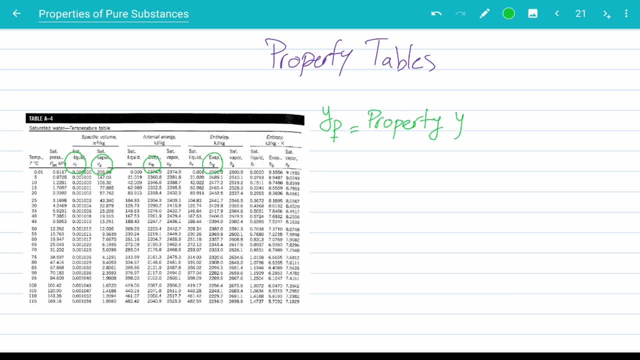 represents the property Y of the saturated liquid. Y of G is the property Y of saturated vapor. Y of Fg represents the difference between Y of G and Y of F. So, for example, at the temperature, 25 degrees, Y of F shows the specific volume of the saturated 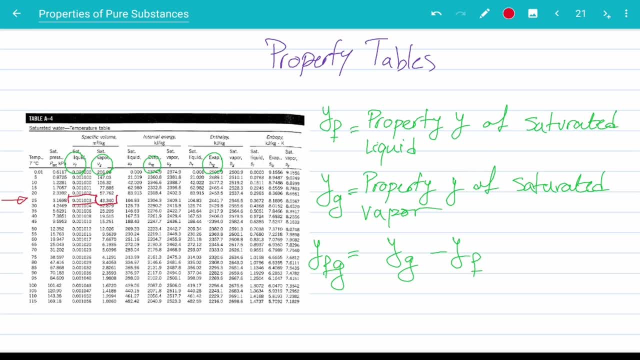 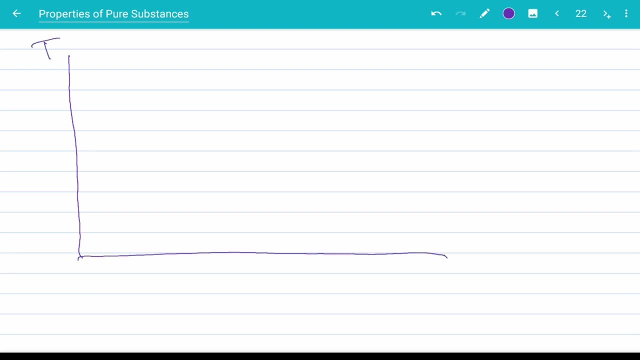 liquid, And V of G represents the specific volume of the saturated vapor. Let's show that on our TV diagram. If this is TV, by the way, TV, TH, TU, TS, all of these look the same. You have the. 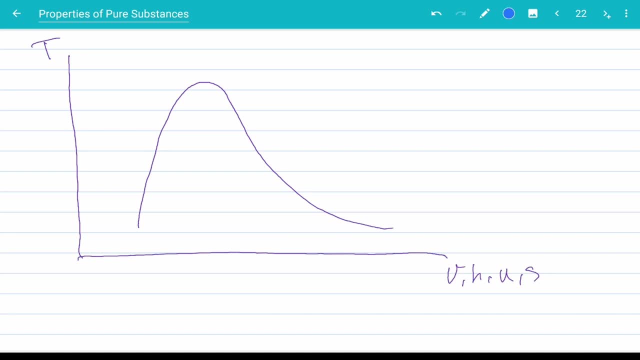 same dome And we have our constant pressure line. So this here is V of F or H of F, or U of F or S of F or whatever. This one here is V of G, H of G, U of G or S of G. This distance is VFG, or H of FG or U of FG. 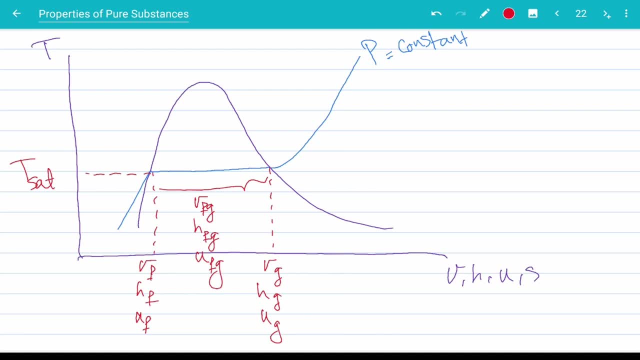 And this is your saturation temperature. Now we have values for this point and this point, but what happens in the middle? Let's talk about that Now. in a saturated mixture, we need to introduce a new property so that we can pinpoint the exact 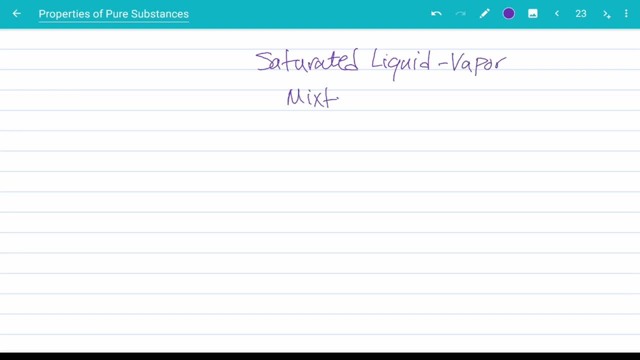 values of specific volume, enthalpy, internal energy and everything else. We call this new property the quality of the mixture. We show it with X and we define it as the mass of the vapor divided by the total mass. So the total mass is mass of vapor. we show it with M of G plus the mass of fluid. we show it with M of F. 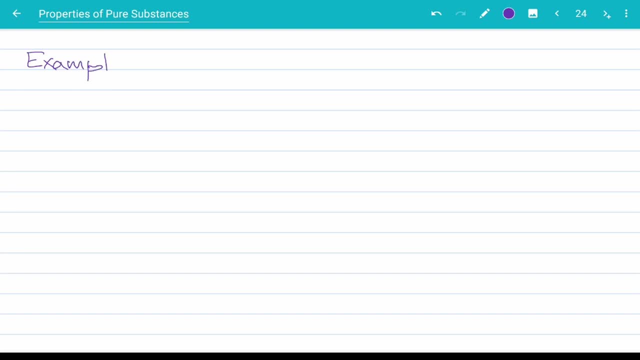 Okay, how does this help us? So let's consider an example. So the volume of a system is the volume of the gas plus the volume of the fluid, When fluid and gas are in a saturated mixture situation. We also know that, mass times, a specific volume is equal to volume. so total mass times, the specific volume of our mixture is: 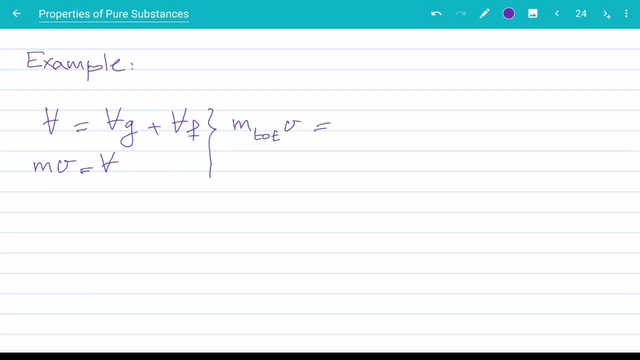 the mass times the volume into M of G of the vapor times a specific volume of the vapor plus the mass of fluid times the specific volume of the fluid. I'm going to divide both sides by the total mass and get the specific volume. is mass of gas over total mass? 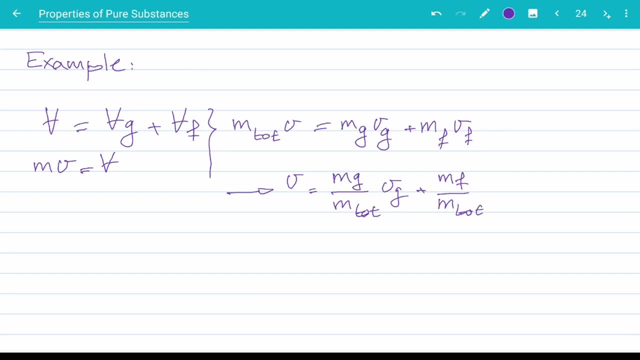 plus mass of fluid over total mass times a specific volume of the saturated liquid. Now do a bit of algebra and we get x V of G plus 1 minus x V of F. We can rewrite it into this equation. At this point, our vanishing contraptionitty is: 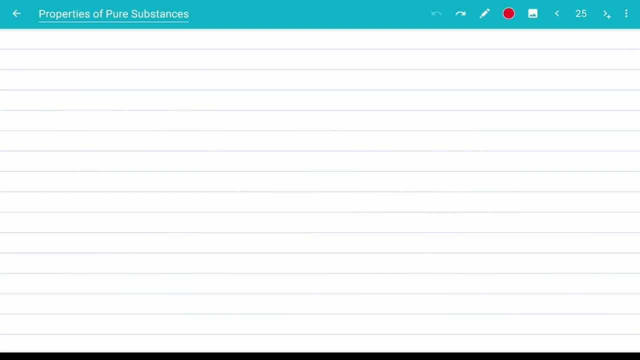 of a larger value. So, just to recap, In a saturated mixture, any property can be found using these equations. So what does this X show? So, if this is our TV diagram and this is our constant pressure line, This shows x. Now, one thing to keep in mind is that, because x is the mass of vapor over the total mass, 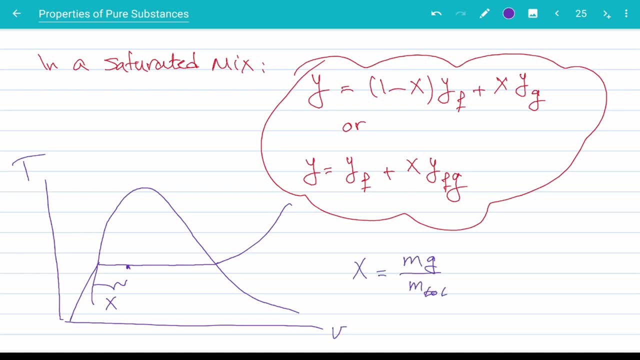 it has a range of zero, and one Zero is when the system is in saturated liquid form, And one is when the system is in saturated vapor form. Another thing to consider is that the y that you get from these equations must always fall between the value of y and y. 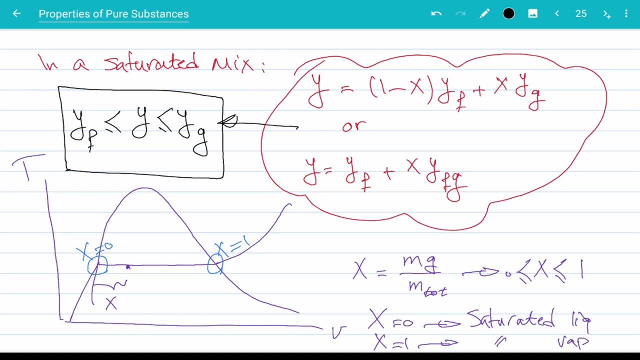 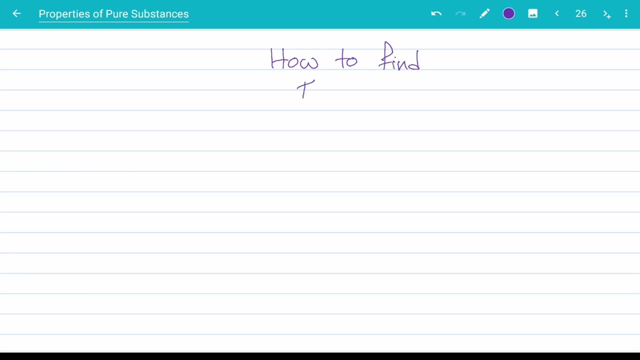 So this is your checkpoint. If you use this equation, find a y which is not in this range, you've done your calculations wrong. Something's wrong. Okay, but how to use these tables? How to find the state of our system? 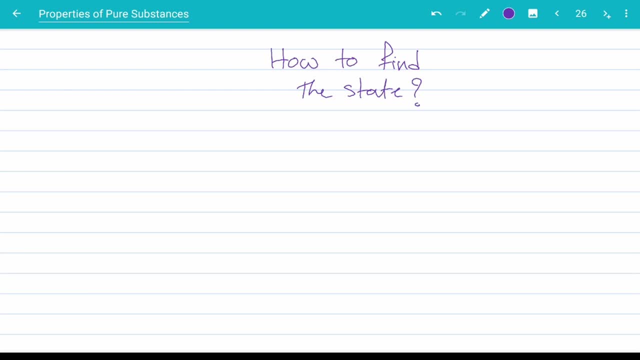 Now it's kind of easy. We just need to remember the state postulate. So the state postulate says we need two intensive and independent properties right to pinpoint the state of our system. Now. intensive, independent properties are the ones that we usually encounter in thermodynamics. 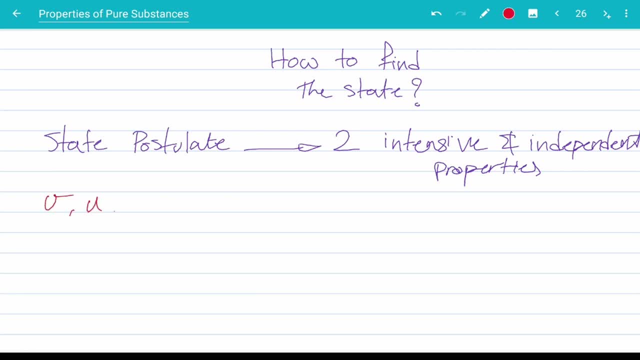 are a specific volume, internal energy, Right, Entropy, entropy- We don't know entropy yet. We're going to talk about it later in later videos- Temperature and pressure And quality for the saturation mixtures. But even if we have two independent and intensive properties, 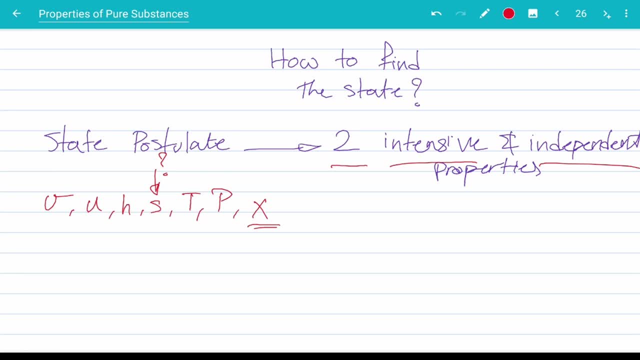 how can we use them with a table? So let's get to it. Let's say you are given the temperature and the specific volume of a system, So you have these two properties. What you can do is you can go check the property tables. 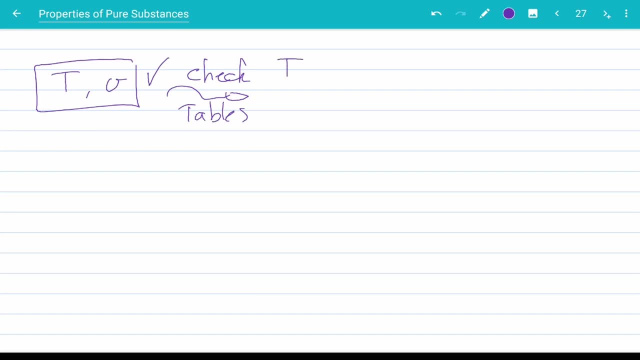 So let's say the temperature is given, The temperature is 75 degrees Celsius And the specific volume of our system is 3.2 meters cubed per kilogram. Right, So these are the two independent intensive properties that we have, And now we want to find the rest of the properties of our system. 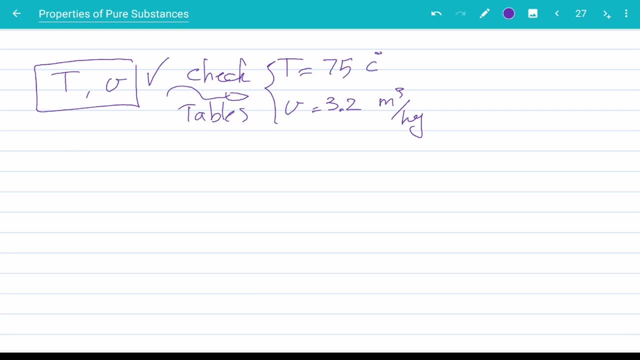 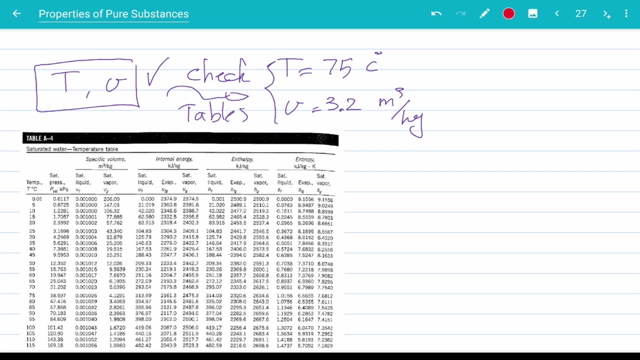 Or in other words, we want to pinpoint the state of our system. So we are going to check the tables. Let's do that, Okay. So this is a property table, Right? I'm going to check the temperature here, So the temperature column is here. 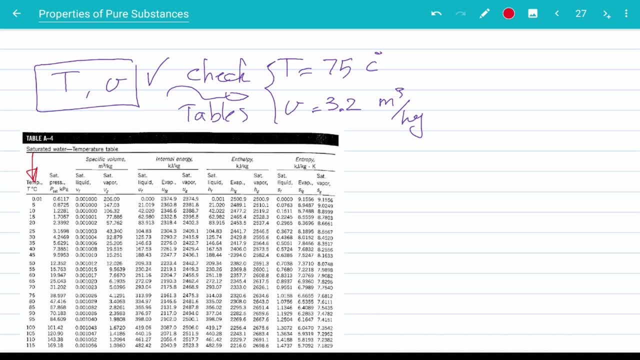 And 75 degrees is here on the table Right. That is 75.. Under the columns of a specific volume of saturated liquid and saturated vapor, you can read two numbers. This is the saturated liquid And this is the number for saturated vapor. 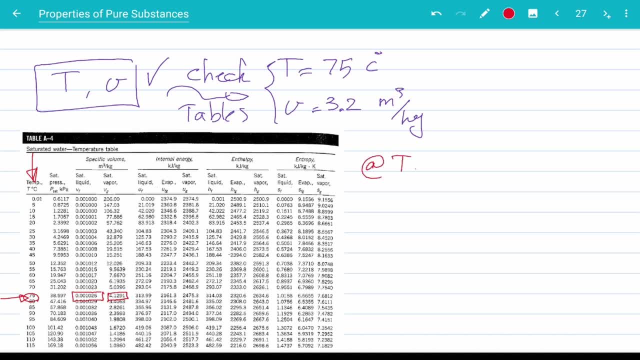 So, at temperature of 75 degrees Celsius, specific volume of saturated liquid is 0.001026.. And the specific volume of saturated vapor is 4.1291,, both meters cubed per kilogram. Okay, The volume that we have is larger than V of F. 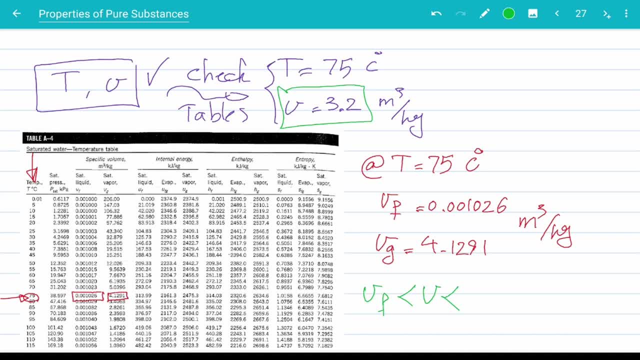 Right, Specific volume of saturated liquid, And is it smaller than V of G or specific volume of saturated vapor. What does it tell you? Let's take a look at the diagrams that we have. So, if this is our T-V diagram, 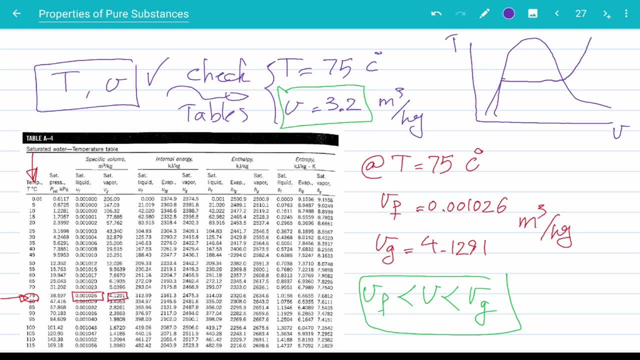 This is our dome And this is the pressure that we are dealing with. This is V of F, This is V of G. The volume that we have is somewhere in between Here. So we are in this area. So we are in saturated mixture area. 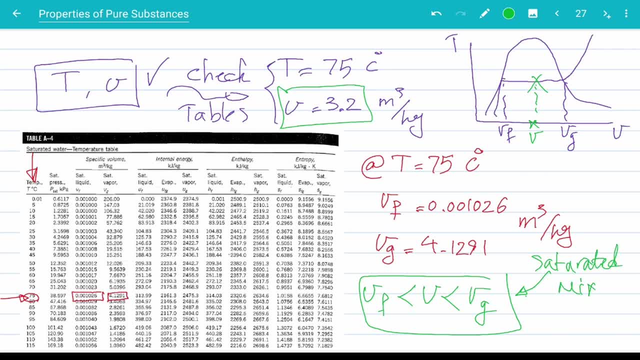 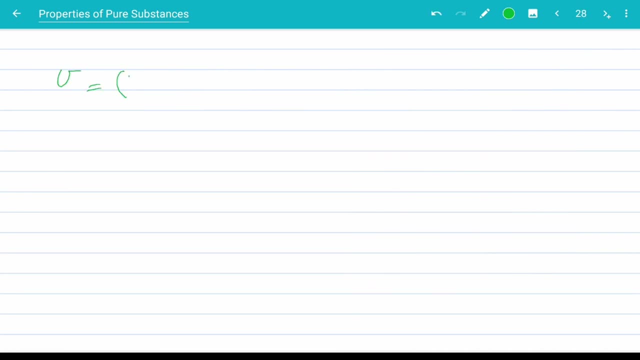 Right Now that we know we are in the saturated mix area, we can find the quality, Always find the quality when you are in the saturated mix area. So a specific volume, Remember, Is 1 minus X, V of F Plus X. 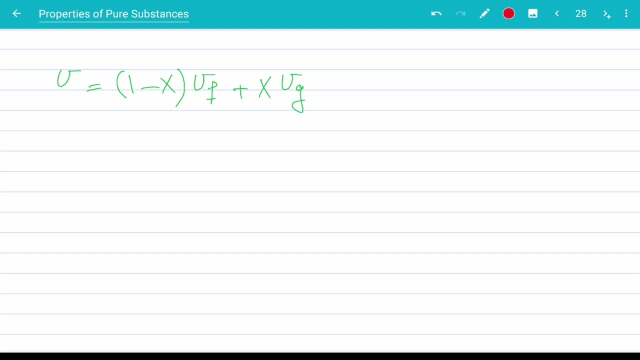 V of G. Now, in this example here, V of F is known Is 001026.. V of G is also known, 4.1291.. Actual specific volume is also known, 3.2.. The only unknown is the quality. 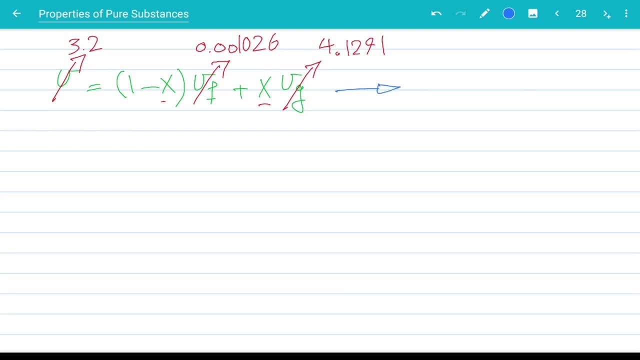 If we do a bit of algebra We find X is 0.7749.. So we found the quality of our mixture. It means we are 77% vapor, 23% liquid in this mixture. Now, if we want to find any other property, 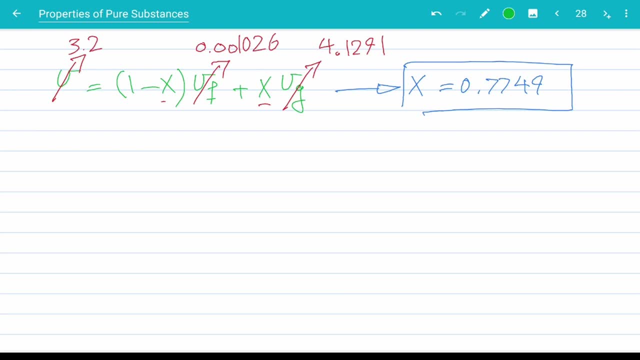 Let's say we want to find internal energy. All we need to do is say: Hey, the internal energy of the mixture Is 1 minus X. We already know U of F Plus X, U of G. Plug in U of F from the table. 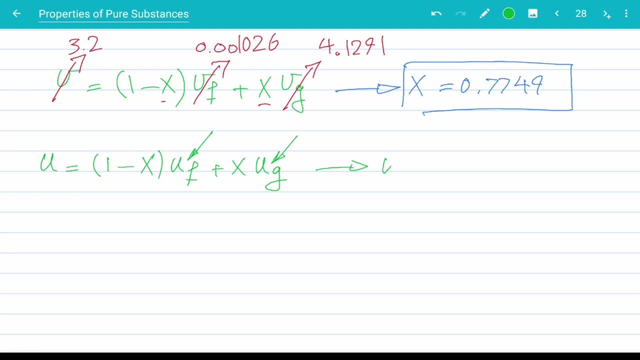 U of G from the table, And we can find U, We can find H, We can find S, We can find all the other properties. One other thing that we can conclude From knowing that we have a saturation mixture Is that 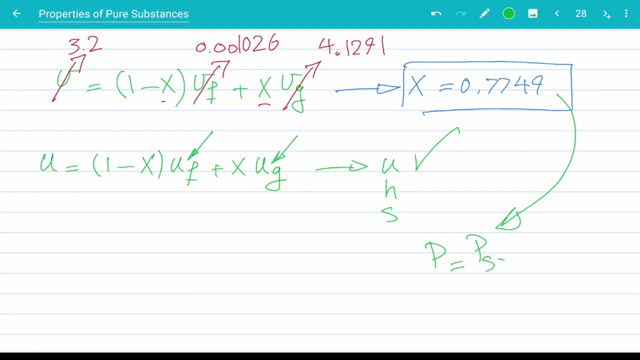 Pressure Is the saturation pressure At T equals 75. Now, because we have a phase change, Pressure is a function of temperature, So all we need to do Is go check the table For temperature of 75 degrees And read the saturation pressure. 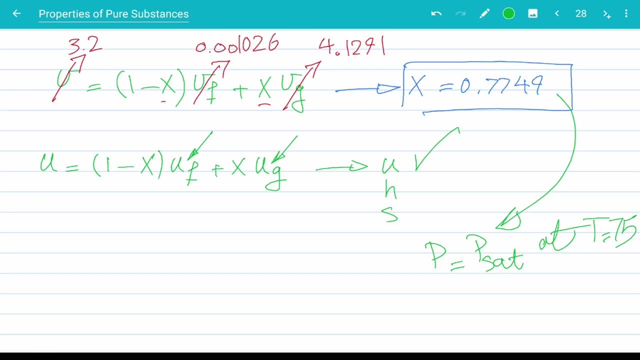 There, By knowing only two Intensive, independent properties, We found all the other properties Of our system. Now what happens If, In that example, The specific volume that we had Was Smaller Than the specific volume Of the saturated liquid? 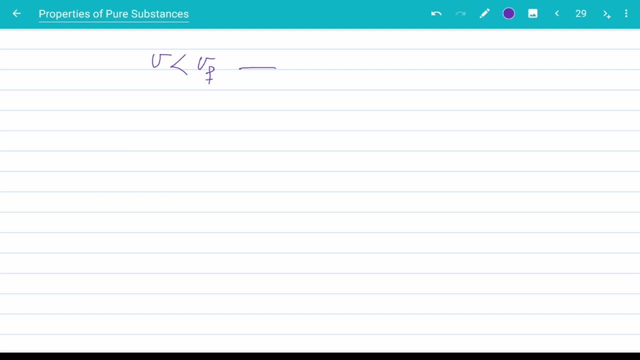 At 75 degrees. Then Let's take a look at our diagram. So this is a, So this is again A T And this is A volume. This is our dome, This is our V of F, This is our. 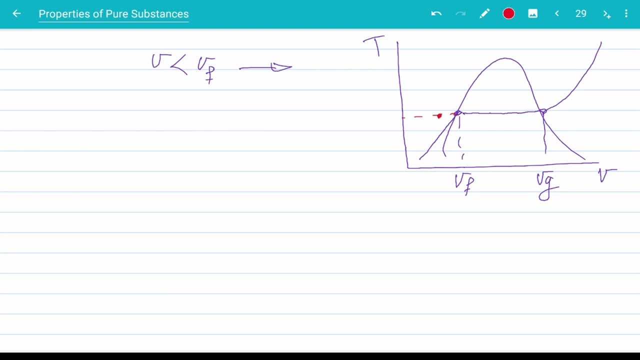 V of G. So we are Somewhere like here Now. this area Is compressed liquid Right. So if the volume Is smaller than the Specific volume Of saturated liquid, We can conclude That we are In the compressed 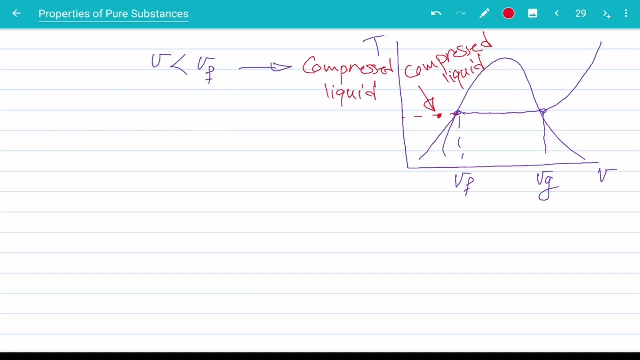 Liquid Area And go Check the table For compressed liquid. If Our volume Was larger than The specific Volume Of saturated vapor, We would end up Somewhere like here, Which is the superheated region. 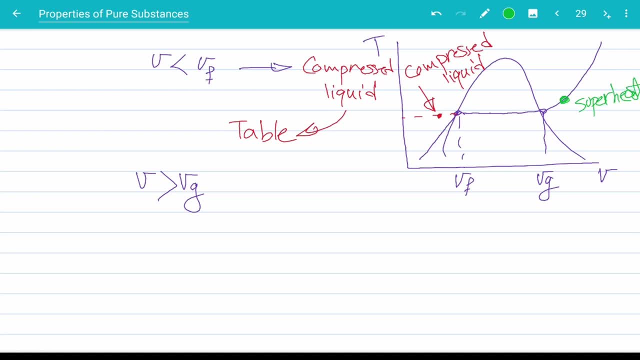 Right, So We would conclude That if V is larger than V of G, We are in the superheated region, And we would go Check The table For superheated Properties Now. please take note. 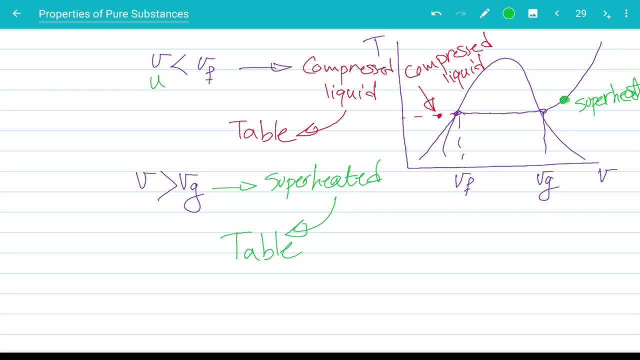 That the volume Can be replaced By U Or enthalpy Or even entropy. So If V is larger than V of G, We can conclude That we are In the compressed Liquid Area And go. 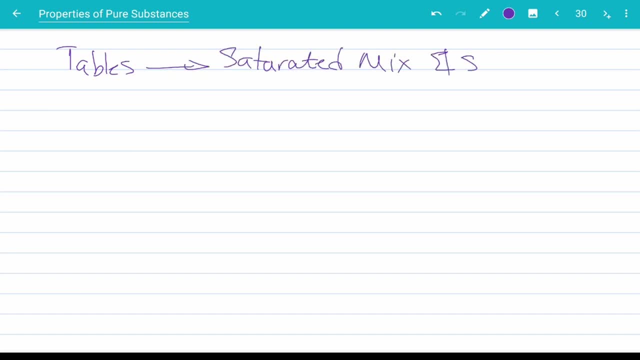 Check the table For saturated Mixture And superheated Regions. Now, Usually There are Tables For both Saturated Mixture And superheated Regions. There are Also Tables For compressed. 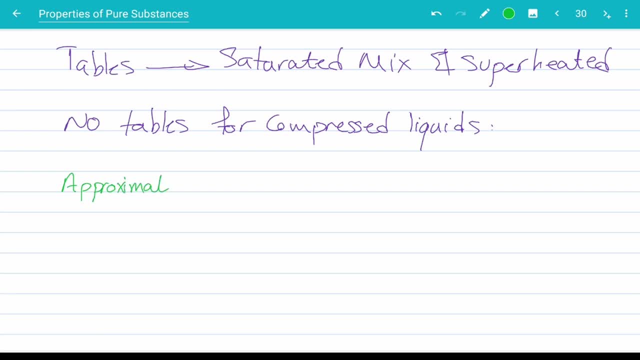 Liquid. Now We are going To approximate, Now We are going To say: The property That we are Looking for For compressed Liquid Is Approximately Equal To the Property Of saturated Liquid. 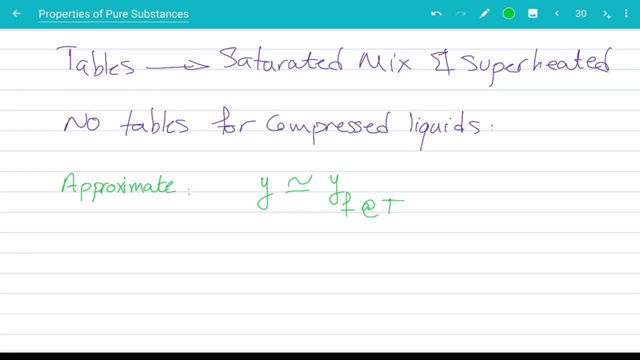 At the same Temperature, Right So, Because We don't have A table Dedicated To compressed Liquids Most of the time. Sometimes What we do Is We read The temperature, We decide That. 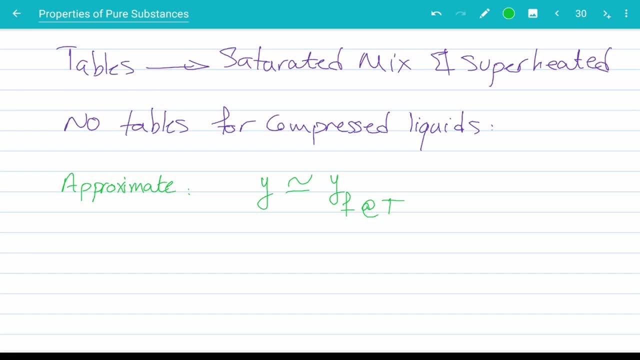 Hey, If we are In the compressed Liquid But We don't have Enough Data, We are- We go And read The property At the same Temperature For saturated Liquid And take It. 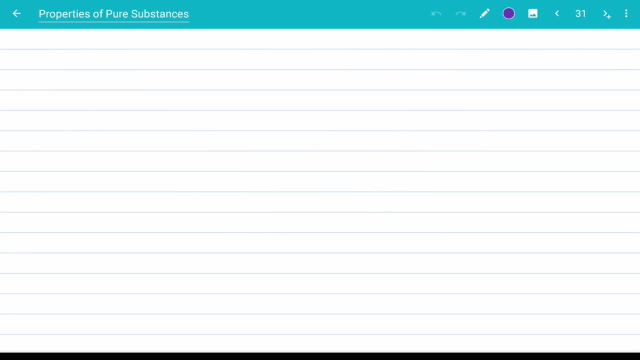 As The property Of our Compressed Liquid At the same 25. Meter At the Temperature, All The amount Of Liquid It is I love. Rather 攻 preacher The Net. 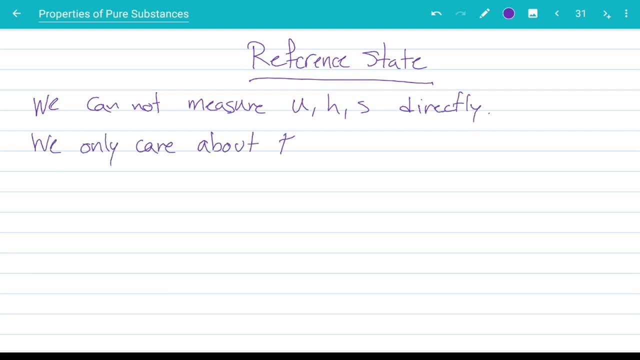 Of Liquid And the Temperature Of ழMn, The Melan, The Temperature At the Start, Annual The is. we can assign a certain state as the reference point and put the values of some of these. 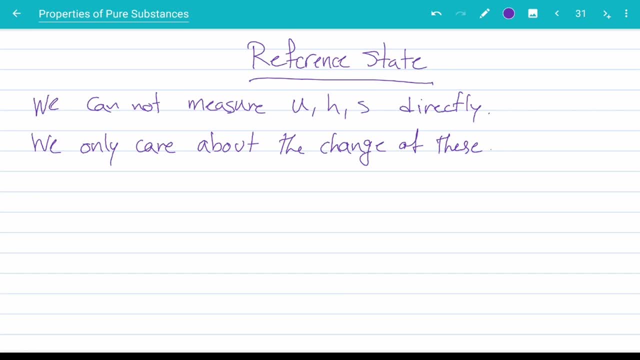 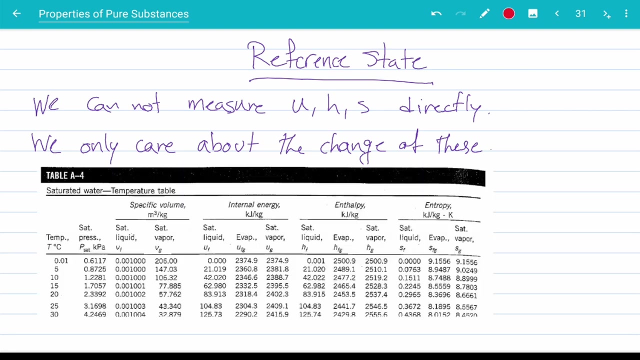 properties zero at that state and then use those equations and relations to build up a value for these properties at different states. Let me give you an example: Back to the table that we had for water at the temperature of 0.01 degrees Celsius and the pressure of 0.6117,, in other words the 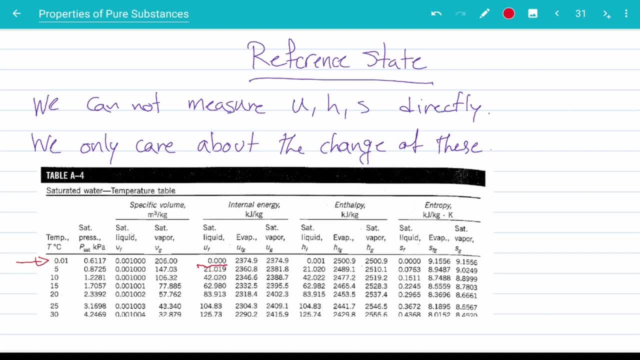 triple point. we are assuming the internal energy to be zero and the enthalpy to be very close to zero. The enthalpy cannot be zero because, remember, enthalpy is internal energy plus p- specific volume. Now, specific volume is a physical property that can be measured directly and as such, it has a 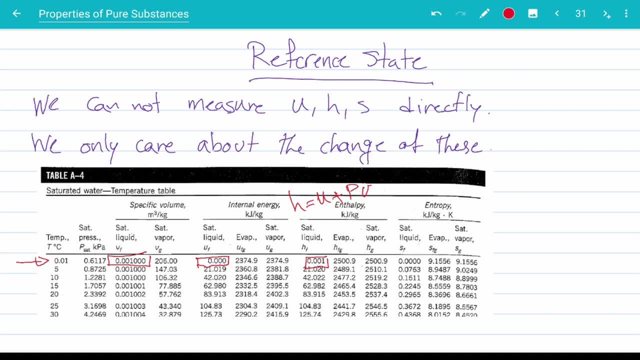 number here, right, Yes, Internal energy. on the other hand, we cannot really find the value directly, So we are going to assign a zero for water at this situation and enthalpy, because of this equation follows to be 0.001 and 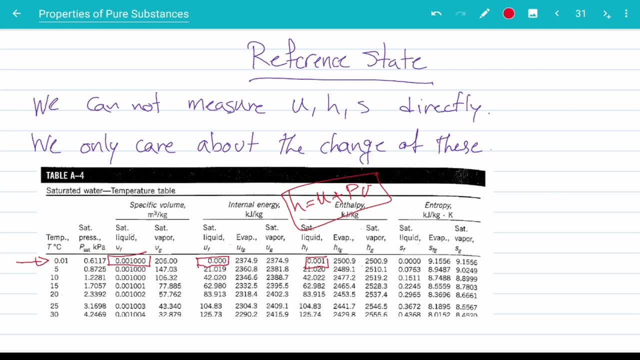 then we build the rest of the table based on this zero value of internal energy. So this is our reference state for water. Now this is how we work. for different pure substances We take different reference states, We assign zero values to some of the properties and then calculate other properties based on the equations. 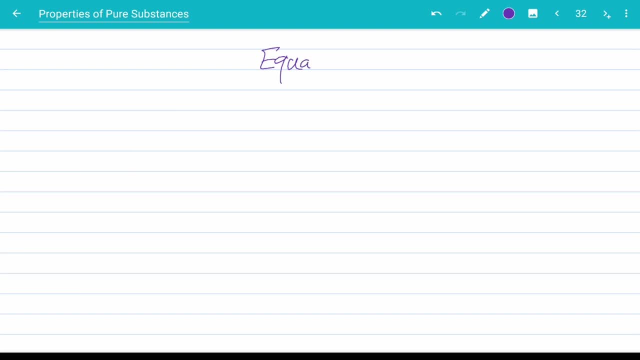 and relations that we have. In many situations, we really want to be able to relate different properties of a system together using a single or simple equation. That will be always easier than using table right Now. unfortunately, not all equations are equal, So you have to use the table to determine the 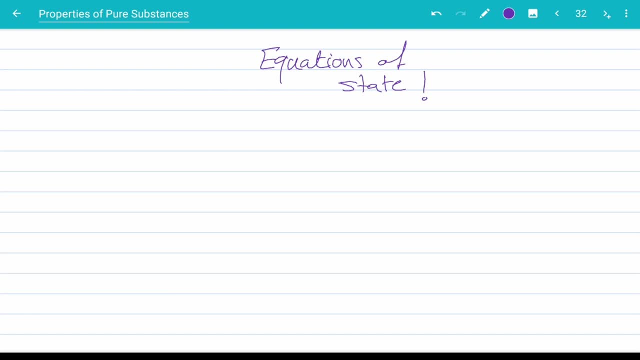 Unfortunately, that is not really possible for most of the cases, but when we are dealing with gases, pure substances in gas forms, especially when we are dealing with gases in low density, meaning high temperatures and low pressures, there are certain equations that can relate different properties of the gas together and give us accurate results. 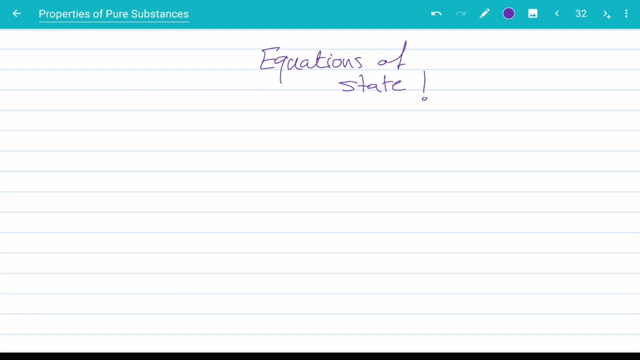 One of these equations is called the ideal gas, which is the most famous form of equations of state, and it says: pressure of the gas times: a specific volume is equal to gas constant times, the temperature of the gas. Now you need to pay attention that this temperature is the absolute temperature. 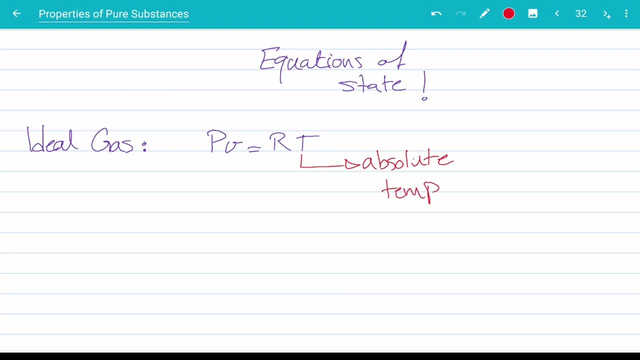 Now, absolute temperature In thermo means temperature in Kelvin. Now, just to refresh your minds, Kelvin temperature or Kelvin scale is the centigrade plus 273.. So water boils in 100 degrees Celsius, which is 373 Kelvin. Okay, That's the conversion rate that you need to use. 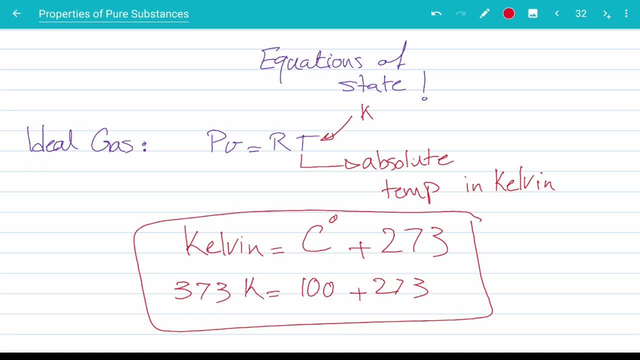 So here make sure that you are using Kelvin. So R is the gas constant. How do we find it? R for each gas is the universal gas constant divided by the molar mass of gas. Now, what are these? The universal gas constant is 8.3.. 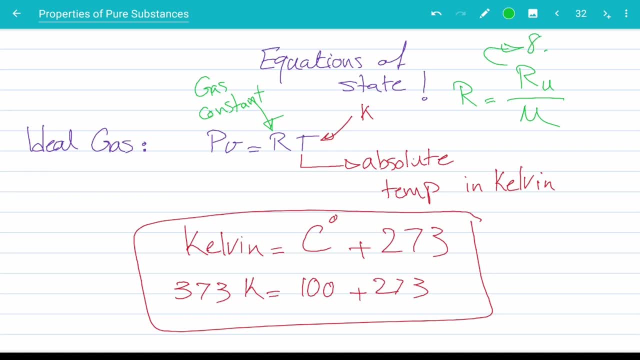 Okay. Okay, So the universal gas constant is 8.31447 kilojoules per kilomole Kelvin, whereas the molar mass is different for different gases. Molar mass is the mass of one kilomole of gas, For example. 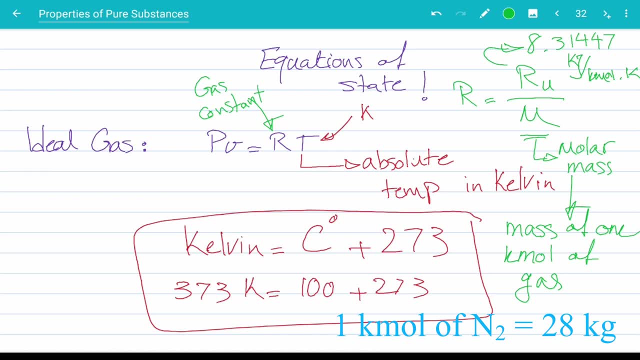 The mass of one kilomole of nitrogen is 28 kilograms. The values for the gas constants are usually given in tables, So don't really worry about the molar mass and the universal gas constant and things like that. Usually the R or the gas constants are given. 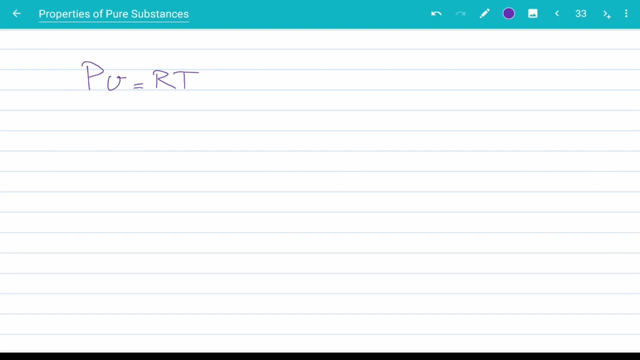 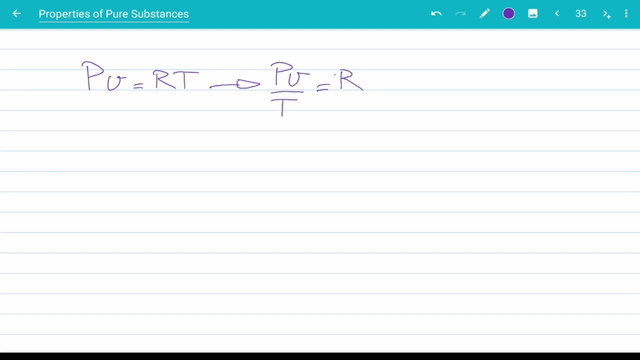 And then say: okay, R is the constant, So PV over T is a constant right. So from this equation, writing it for two different states of the same gas with the same mass, we can conclude that P1- V1 over T1 is equal to P2- V2 over T. Now this is a 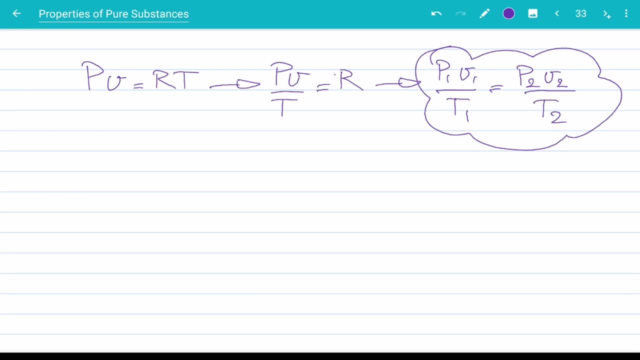 very important conclusion. Now for the same gas in the same system. we can always use this equation to relate the different properties of the gas at state one to state two. We can write this equation in other forms as well. We can rewrite it in the form of P1 times the actual volume one. 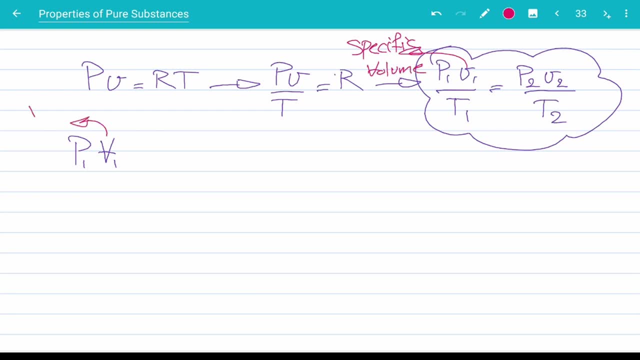 This one was the specific volume, whereas this one is the volume. Now, as I said, ideal gas is a constant, So we can write this equation in other forms as well. We can rewrite it in the form of P1 times the actual volume one. 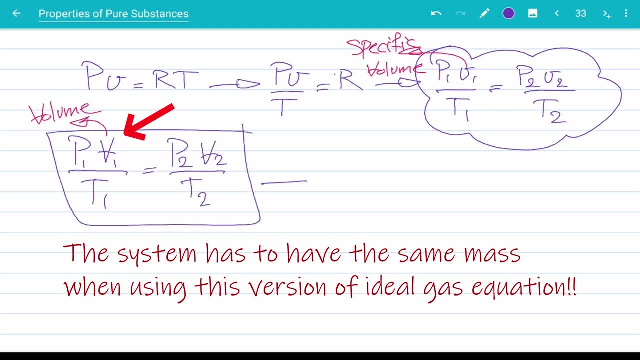 This one was the specific volume one, So we can write this equation in other forms as well. We can rewrite this equation in other forms as well, So in other forms. as I said, ideal gas is a constant, So P1 over T is a constant. 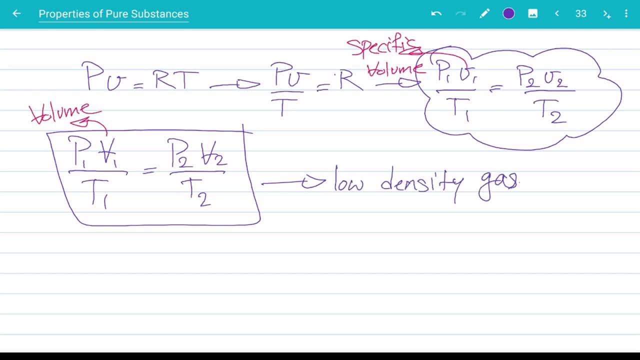 So we can rewrite this equation in other forms as well, And we can rewrite it in other forms as well, And so the ideal gas equation is giving us very good results when dealing with low density gases, meaning usually high temperatures and low pressures. In these situations, the ideal gas equation is very good and very accurate. 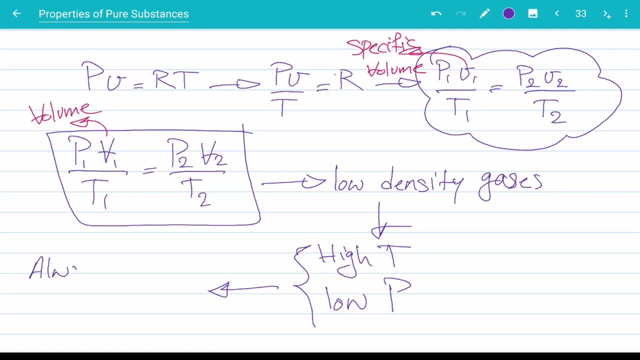 Now for our applications in thermodynamic course, we can nearly always use the ideal ideal gas equation for air. Okay, so whenever we are dealing with air, with oxygen, with nitrogen, with carbon monoxide, carbon dioxide, we can always use the ideal gas in thermodynamics. 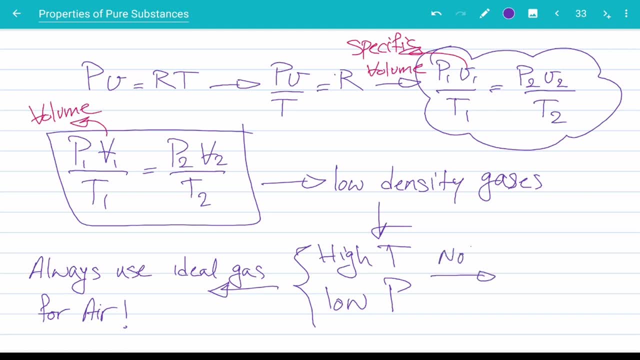 On the other hand, we cannot use it when dealing with substances that usually undergo phase changes, like steam or water vapor. Never use it with steam. Never use it with refrigerants- Like we are going to talk about refrigerants and refrigeration cycles and such later- but a